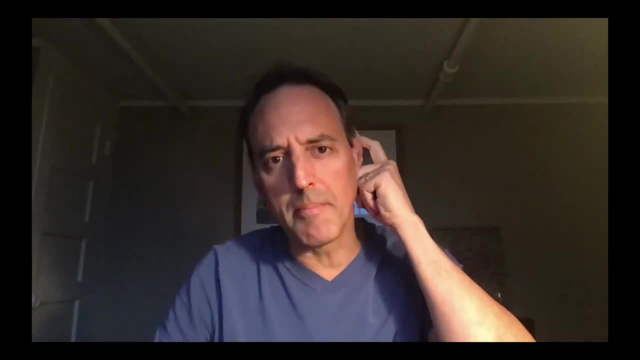 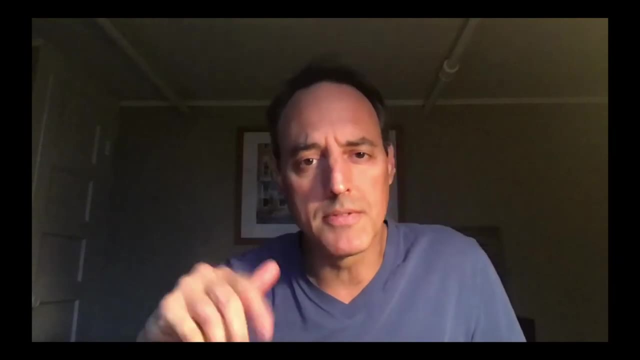 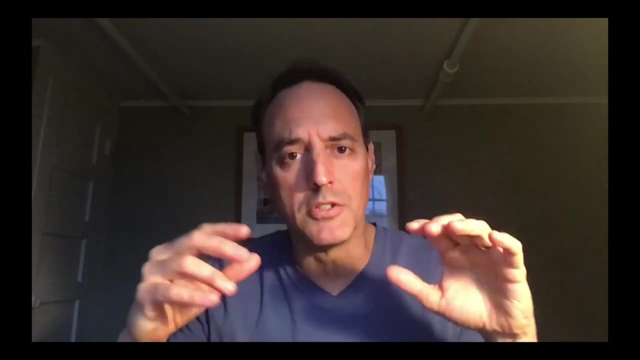 and then we're going to do a little demonstration on MATLAB and the use of these in MATLAB and also show you some of the functionality that these iterative schemes offer you in terms of looking at its convergence properties, dictating the iterations, dictating the convergence itself. 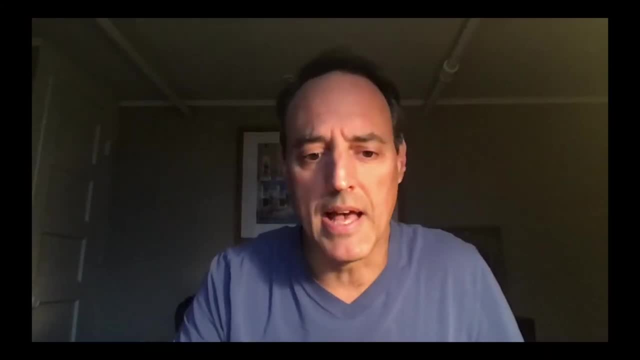 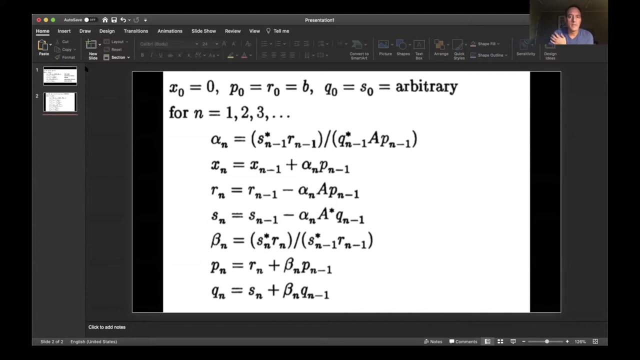 So I will certainly highlight that as we go through this. Okay, so first of all, let's talk about it from the point of view of an algorithm- and I'm going to go and share screen here- and the algorithm, kind of interestingly enough, is: um, there we go, start here. the algorithm itself starts off with some 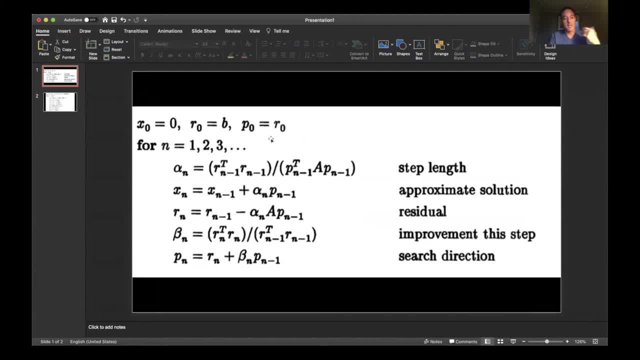 initial guesses. so this is the idea you're going to start off with it. you're going to solve a x equal to b. you're going to start off with an initial guess, which is here: x naught is equal to zero, and what you'd like to do is you pick a residual, you guess a residual which is going to 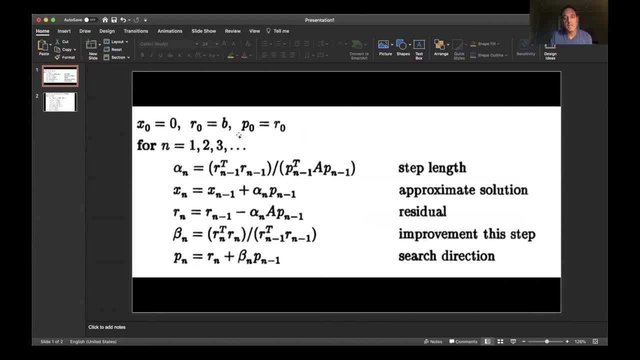 just be b itself. and then you pick this other vector, p, which in some sense is going to look a little bit like the search direction in gradient descent. so that's why it's called gradient conjugate gradient methods. Okay, so we're initially going to pick the p to be r zero, which is 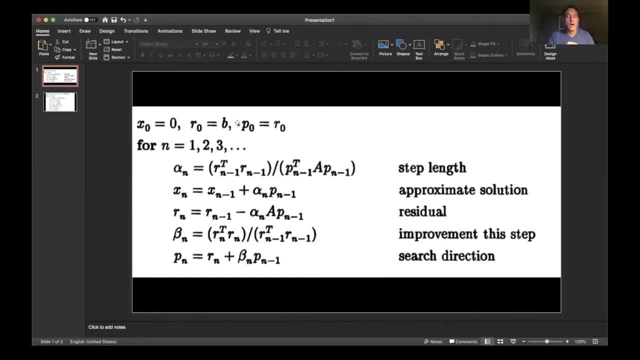 b. so this is our initial guess. remember that in some of these kind of algorithms like Jacobi or Gauss-Seidel, if you have a strictly diagonal dominant structure, you're guaranteed to converge, no matter how you guess this. so, but these are the initial guesses, and then you go into the loop. 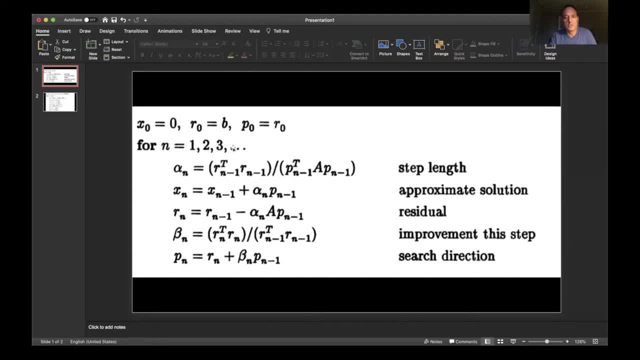 So the first thing you do is you start to pick a direction to search in. so the idea here is to take r zero transpose r and p zero transpose a p zero. so notice that this p zero transpose a p zero looks a lot like the Rayleigh quotient right. so it's projecting onto that matrix a and giving you 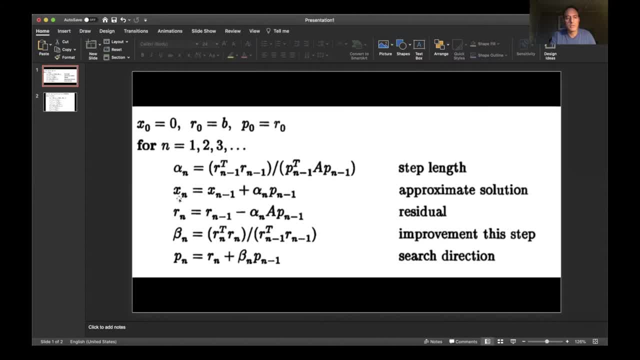 a direction. and then what you do is you approximate the solution x of n is your current value plus this alpha value times the p, and you take a step and then, with this new value, you calculate the residual. the new residual is the old residual plus. here you go, you calculate a acting on p of n. 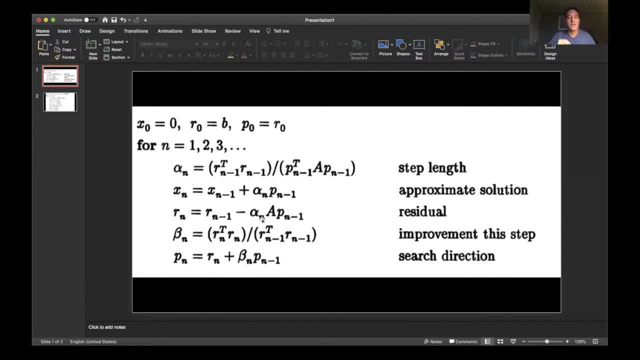 times alpha of n. so this gives you in some sense a step in the residual direction, and then you look at the improvement of how you've done. remember that r is sort of supposed to be like a residual, so you can compute your r of n, transpose r of n versus r of n minus one, r of n minus one. so 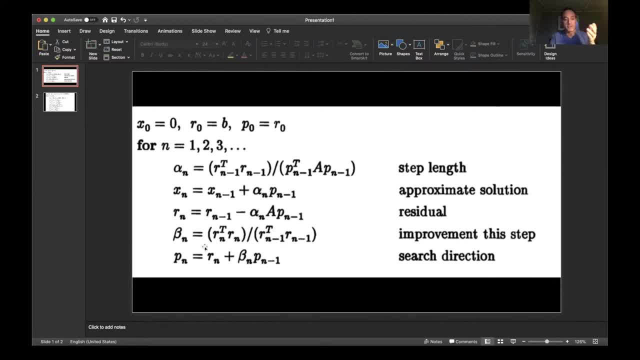 presumably, as your rn is getting better, this beta n is getting smaller, right, so that's that's the idea, is that you should be improving, and then you change your search direction. your p of n is what the r of n is times this b of n, p of n minus one, so it's kind of defined as just an algorithm. 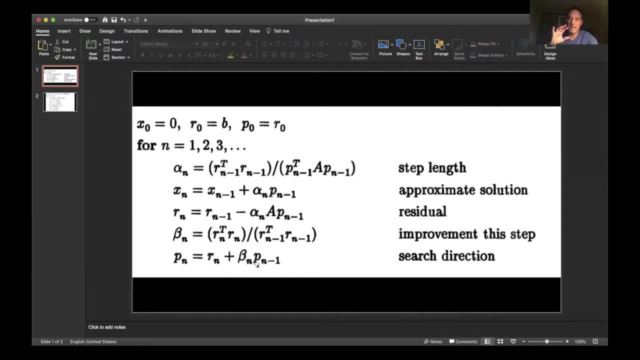 that if you kind of spend some time and you dissect back what these things are you're going to be doing, you can make sense of each of the steps, um, in terms of a search for a solution. so this con, it's called conjugate uh, gradient, descent uh uh, and so. so this is uh part of what 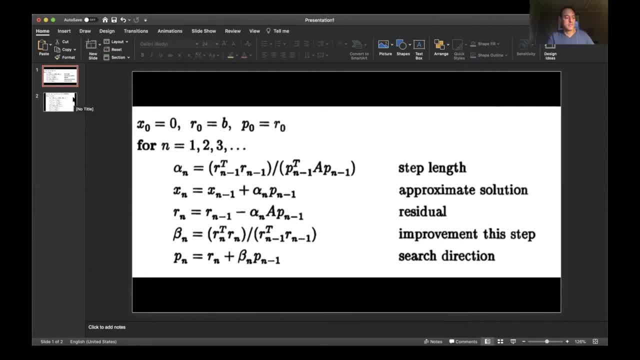 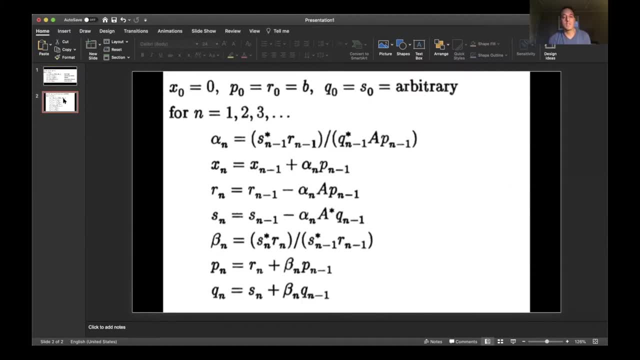 you want in terms of uh, in terms of looking for solutions and iterative structure. a more uh, a broader class of this is when you have uh, just you're just searching in your solutions can be complex, uh and uh. and there's no restrictions on matrix a and this is called. 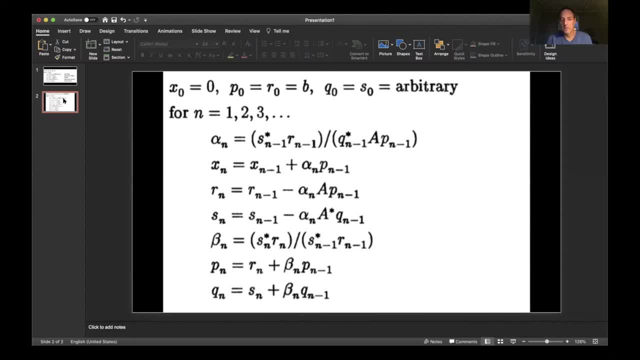 biconjugate gradient descent: very similar. but instead of working with just r and p, we're going to actually work with two sets of vectors: p0 r0, q0 s0, and this is how you pick them. so the p0 r0, just like the before with b, and q0 s0 are arbitrary, and notice what we're going to do here. 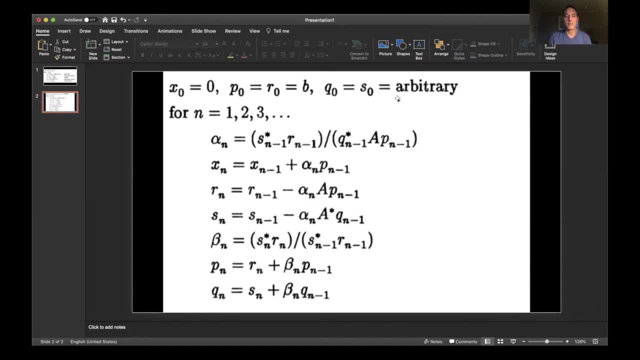 is, we're going to have left and right multiplies in this algorithm, so you're going to define a length again for the iteration step, which is now though projection onto s and q, which are these arbitrary vectors, and again forming some kind of inner product with a Rayleigh quotient, and then you update your values. x of n is what it was before. 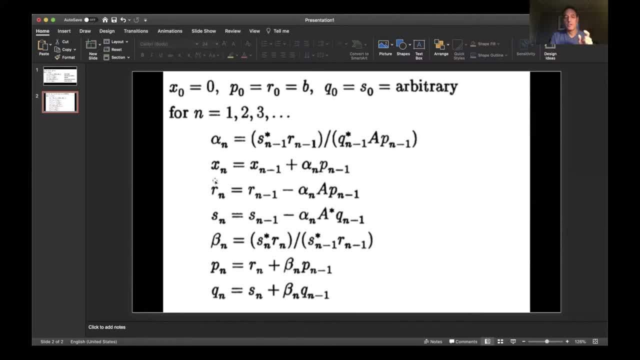 plus the search direction times: p of n, update your residue residual, update your s of n, b of n, p of n, q of n. so you just update them and just iterate progressively and each of these sort of has a little bit of the structure like a gradient descent. but now it's this: using this dual vector spaces of the q's, q, s, p and r, 0 to 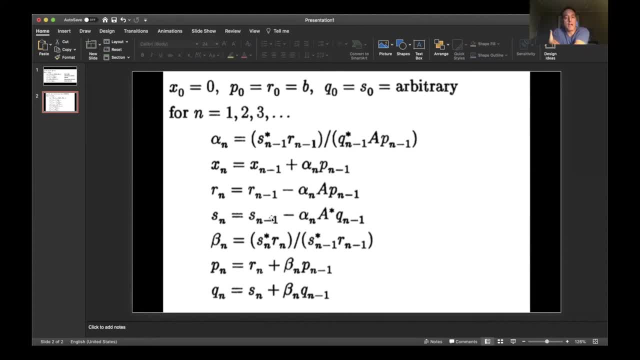 search in this space and notice that you have complex conjugation explicitly in the algorithm. so this is kind of the structure. there's actually a lot here of details again that we are not going to get into around gradient descent methods or by conjugate gradient descent methods. what we're going to do really is: 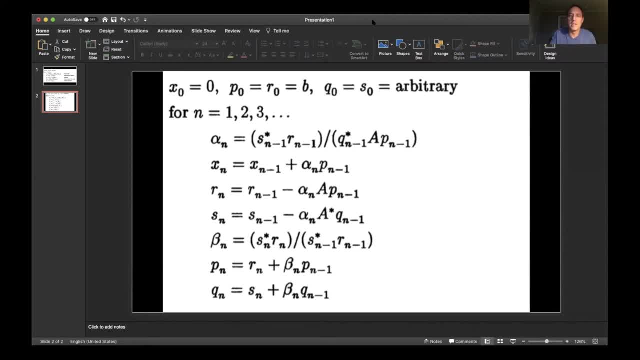 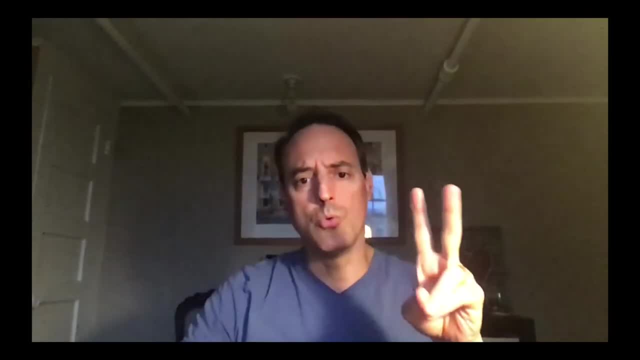 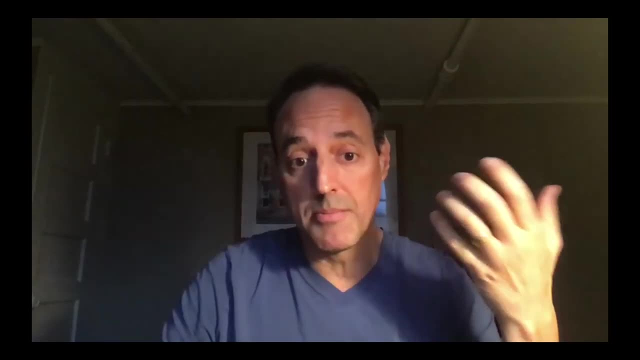 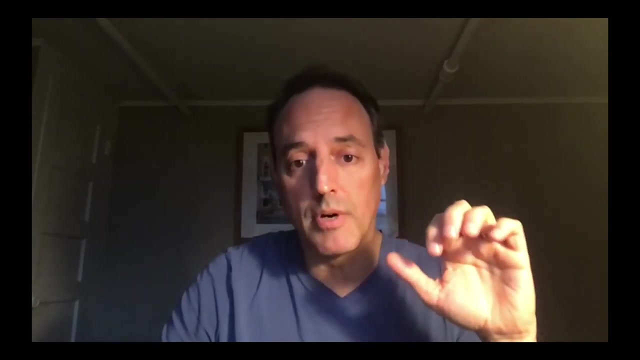 just come back to thinking about MATLAB and implementing this in MATLAB. so, without further ado, what I want to actually do is talk about two algorithms in MATLAB that implement these things. one is the GM res, the generalized method of residuals, which I talked about in the last lecture, and now this one is- and also I'm going to talk about- by conjugate gradient. 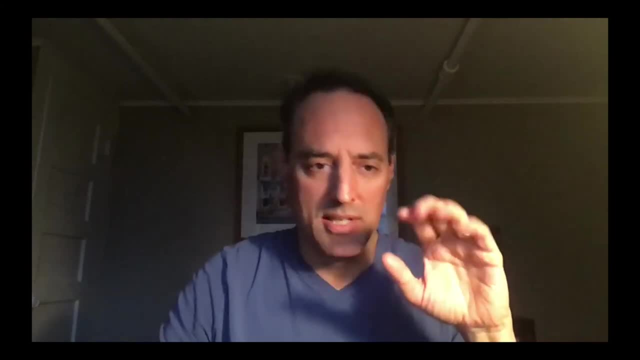 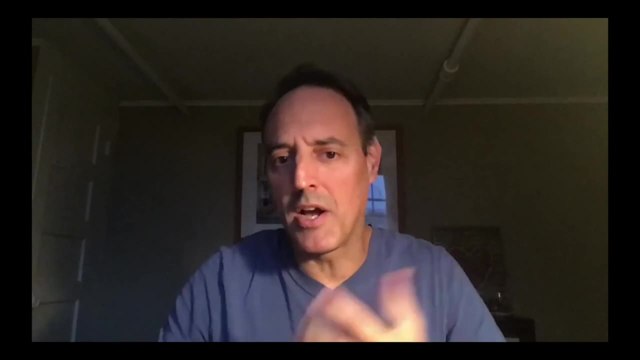 so I'm going to talk about a stabilized method by cg stab. so it's like what the algorithm, second algorithm- I just showed you, except for there's some stabilization steps in there as well, so these get quite complicated. but again, remember you're, all of this is aimed at beating the 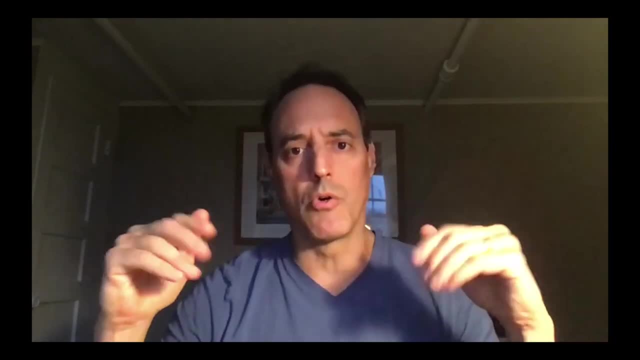 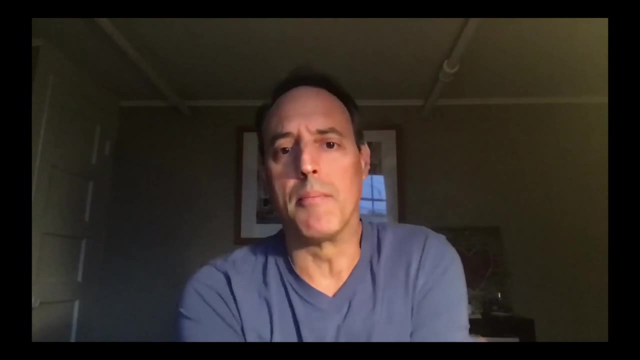 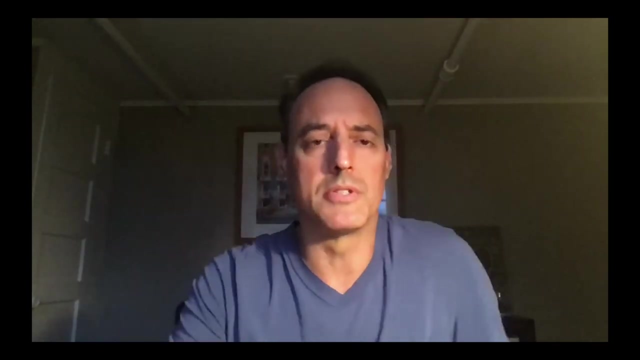 bottleneck of order n cubed, right. so that's our bottleneck that we're going after. how could I solve an ax equal to b for a very large system faster than order m cubed? because that's that's. uh, if that's what you're solving it in, it's extremely slow, especially for large matrices. 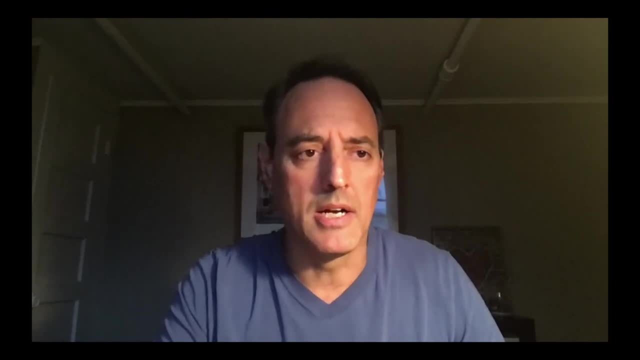 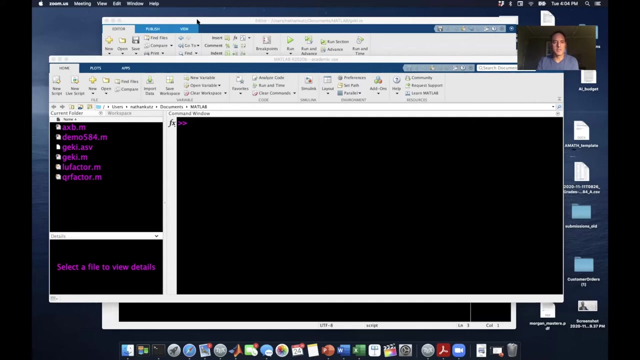 all right. so with that in mind, let's go and, uh, go ahead and start looking at some MATLAB here. so I'm going to share screen, I'm going to program in MATLAB, all right. so here we are, we're in MATLAB and we're going to start programming this. the first thing I want to do is just do a help. gm res. 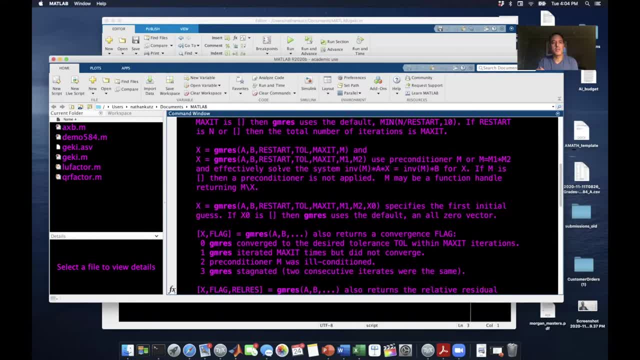 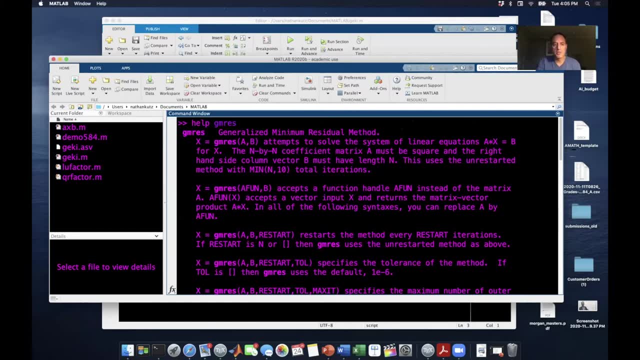 that's the command we want to look at. so here we go. so gm res. so bring it to the top here: generalized mythum, minimum residual method. so gm res. all you do is say, if I have a matrix ax- sorry, matrix a and a, b, I have ax equal to b. I put a and b here, it gives me a solution: x in fact. 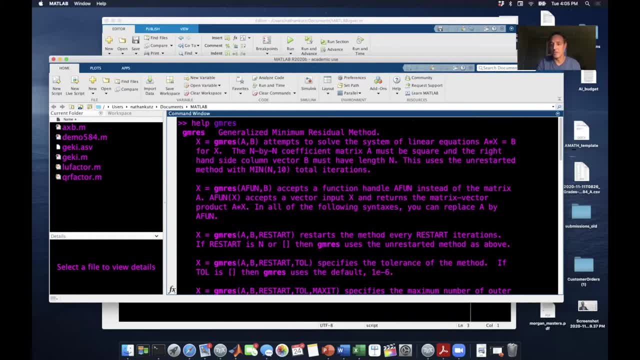 notice what it says: attempts to solve the system of linear equations x equal to b. okay, so that's what you're going to go after. is you're going to actually go ahead and put this in and it's going to iterate, using that gm res algorithm, towards trying to iterate towards? 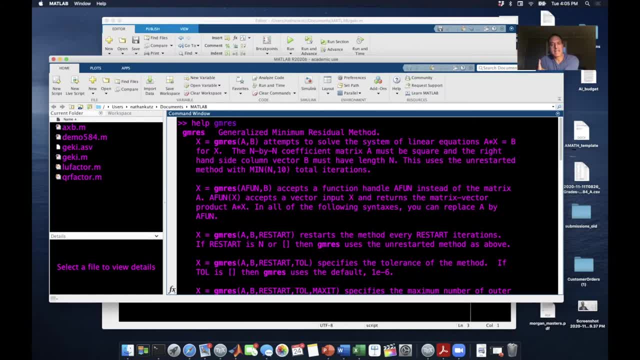 solution: convergence. I'm going to give a very bad example of this here. I mean oftentimes, when you structure these matrices, a, like as I made a comment in class a, oftentimes has is large and diagonally and has sort of sort of almost a diagonal dominant structure so that the iteration. 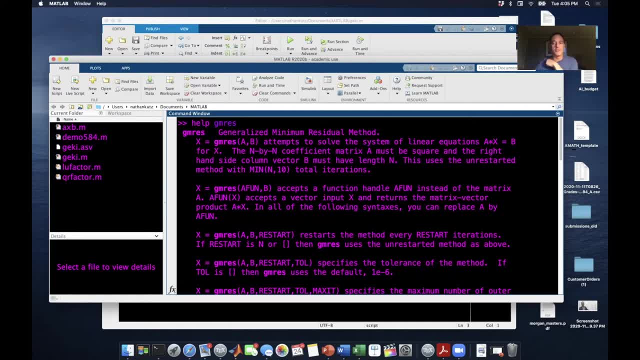 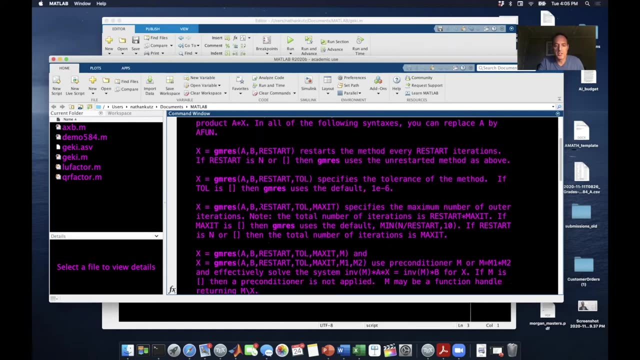 procedure converges very quickly and you'll see here when I do this it takes quite a while to do it. it takes quite a while to converge for just some generic matrix a. I also want to highlight some of the functionalities you get out of gm res. it's all listed here. but you can take gm res and let me 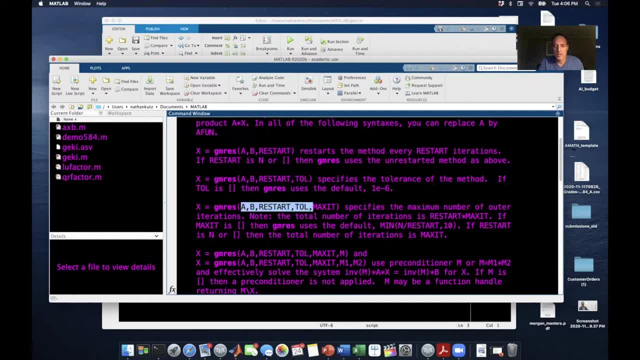 come down to here and you give it a and b and this is this line of code, right here. right, so you can give it options, you can have it restart. in other words, it's going to iterate a certain amount of times and stop and you can restart it. okay, you can specify the time that you want it to start. 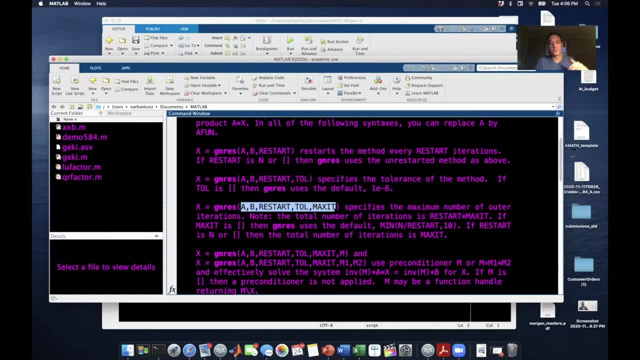 and then it will just submit the itself. so I'm going to start the iteration in the way that it should start. so I'm going to start that and I'm going to say, um, yeah, all right, so that's the way that it can start, and then I'm going to say, well, I'll just give it a little time to wait. 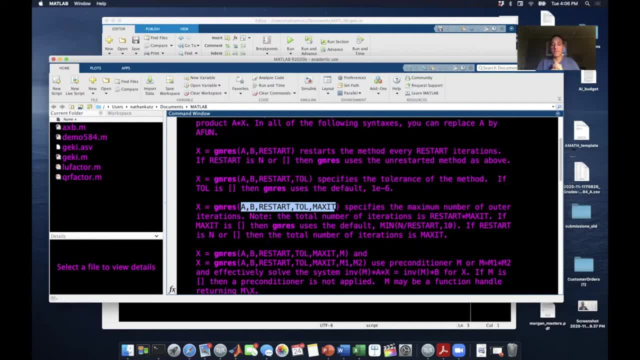 and then I'll just stop and then we can see pretty fast how this is going to work. so what it's going to do is it's going to take 10 iterations and notice that it's going to stop if I fit it in at 10. and in this case it's going to take 10 iterations and then, when it's, 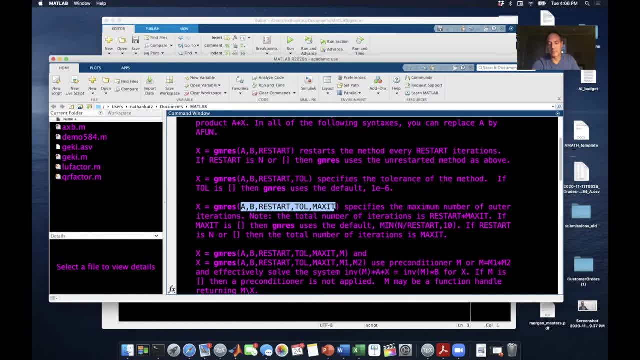 in the max number of iterations you're going to see that's a little bit different than that: a solution within 10 iterations. and so there's reasons why that would work, because oftentimes you're solving this ax equal to b, where b changes slightly, so you have a solution for x equal to b. 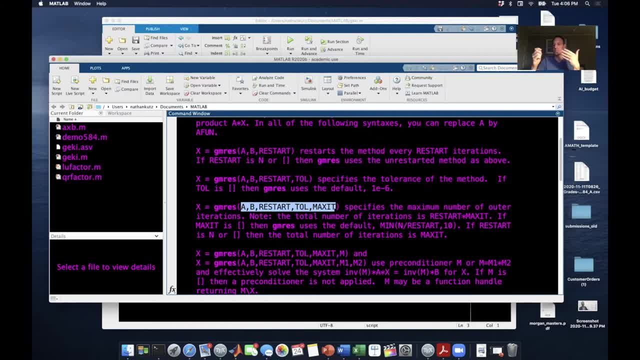 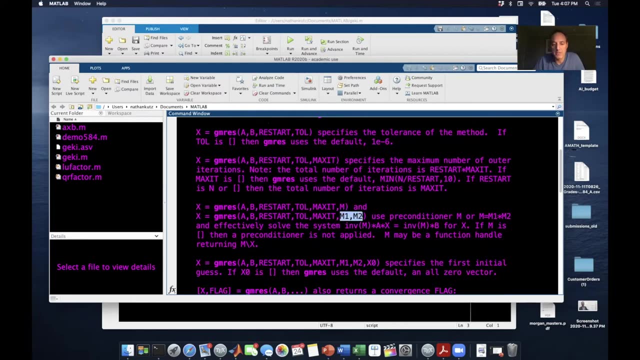 and b changes slightly, so all you need to do is update that solution, so you use your previous solution for this, and this often happens when solving partial differential equations. there are other options. you can even bring in what are called preconditioning matrices. uh, and one of the things i'll say about this is, again, we've, in some sense, barely scratched. 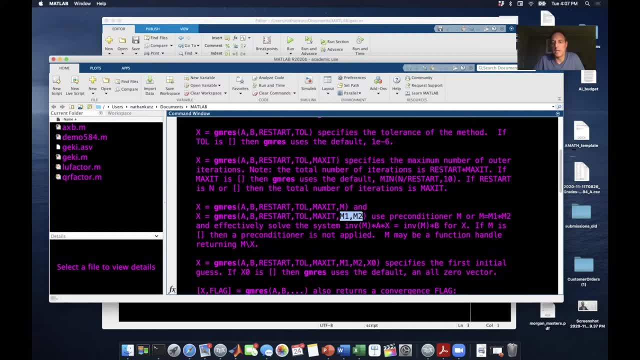 the surface of all the innovations in linear algebra and numerical methods for linear algebra. you were starting to get into the very sophisticated things for solving large-scale systems. but oftentimes there's this idea of preconditioners that can be brought in, which is, ways to transform these matrices to make them a little bit more amenable to the iteration process. 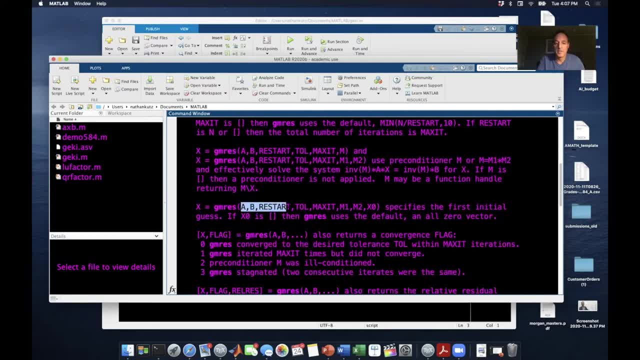 and so, of course, what you want to do is really resonate with the� adding all the DUIs to the model. that would be that mutation phase of the function. so so, in other words, you're taking one X and one of the MCY and you're unlucky to. 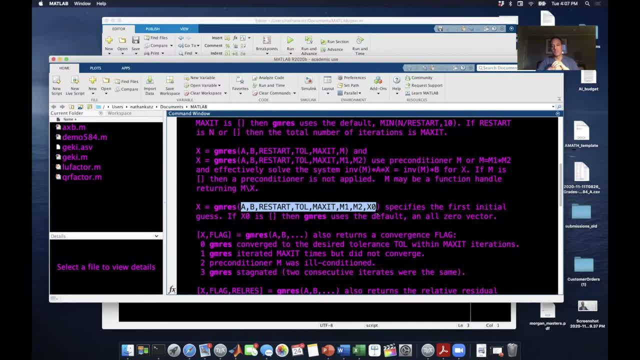 start with one of the equals and lonely, to find this solution that will help you or be useful if you're not go over there and you're lucky to find an integral to this on the part of the process, because otherwise all you're going to do is start adding in these with the 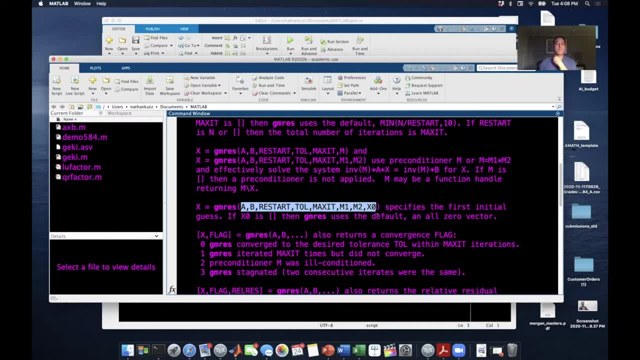 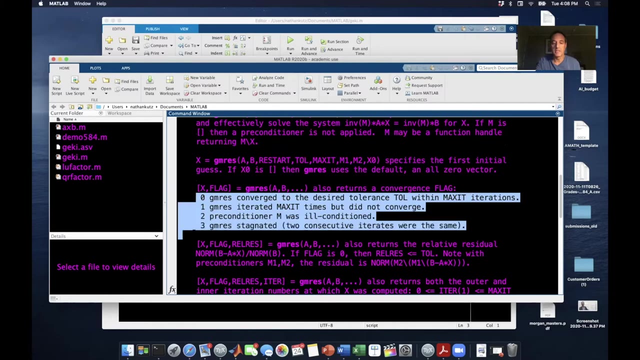 rationmat aberrations. i give a little bit of Yeah, now can just take that closed solution and then make it more accurate. okay, so that's the inputs that you have available to gm res. what about the outputs? well, the outputs can give you a flag. there are different flags that come out of this thing, right, so you know if the flag is zero it. 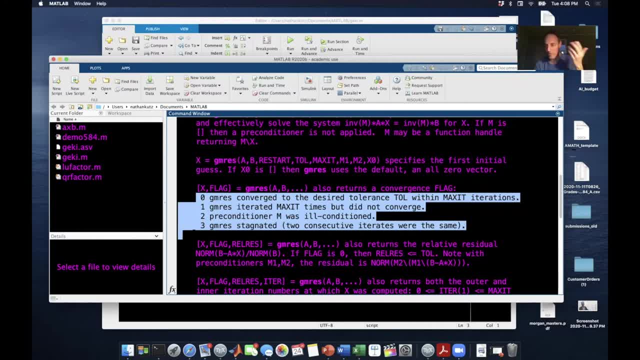 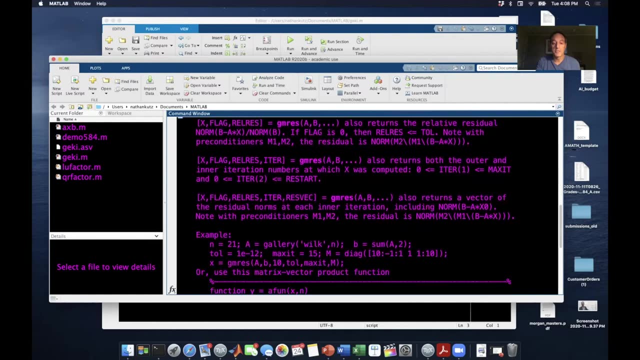 converged, or if one, then it went through the maximum number of iterations and didn't converge. there's some other ones here about ill conditioning of preconditioners and so forth. okay, but really what i want to do is: let's come back to here, because i want to show you this. this is: 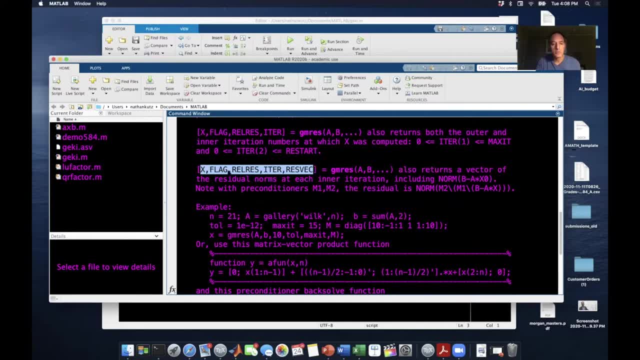 the outputs, because we're going to look at these. i'm going to get the solution x, i'm going to get that flag out, i'm going to get the relative residual. so this is going to give me essentially what my error is. so once i've stopped converging, it's going to tell me what the error is. the. 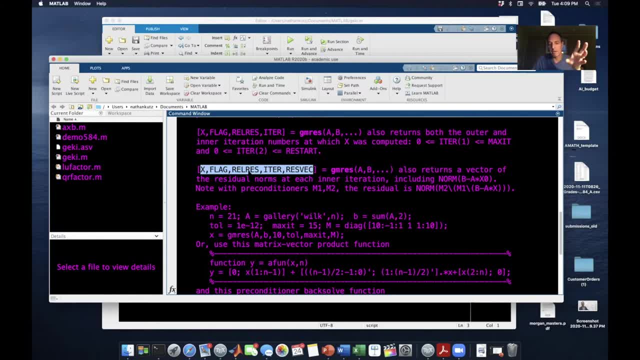 relative residual is going to be. after i stopped iterating, here's your error. iter is the number of iterations says here's the relative you know. so it's going to tell you what the error is and the iteration is like. maybe it took you 52 iterations to get to where you are and that's. 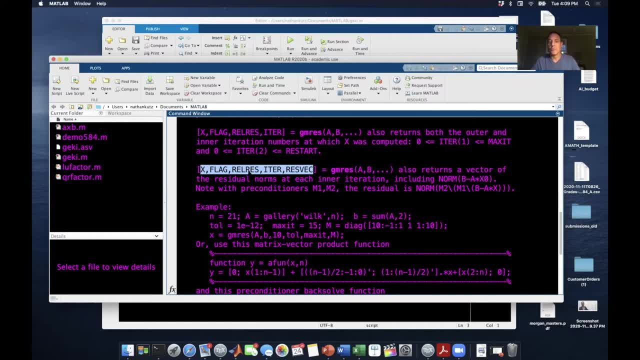 the error, and resvec is a very interesting one. the resvec is a vector of the residuals and we're going to take a look at that. in other words, it's going to keep track at each iteration of how you're doing, and so we're going to explore that one a little bit, because 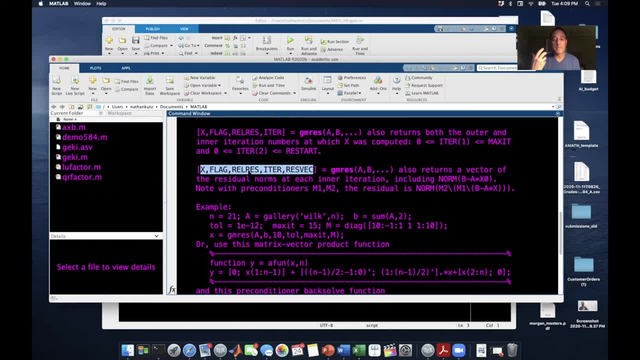 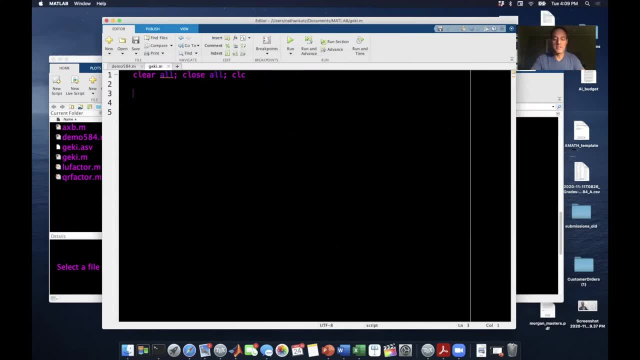 that one's actually kind of fun to look at to see how rapidly the convergence happens for these algorithms. all right, so let's come back to here and let's define a matrix. i'm going to first make this thing 100 by 100, so it's not going to be very big. this is just really just to play around with. 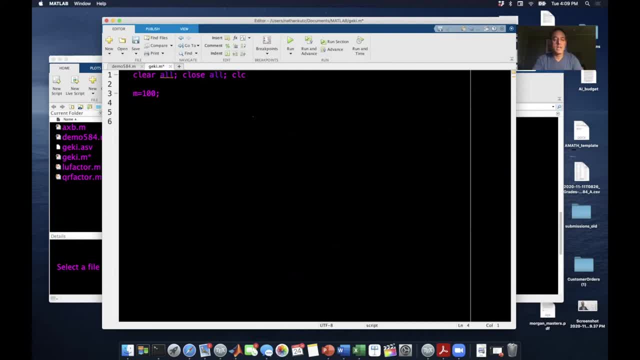 gm rands. okay, and uh, i'm going to say that the matrix a is going to just be some rand matrix, which is m by m, and the b will be some rand vector and by one, and i'm going to go solve this, so, uh, so, first of all, let's call it. 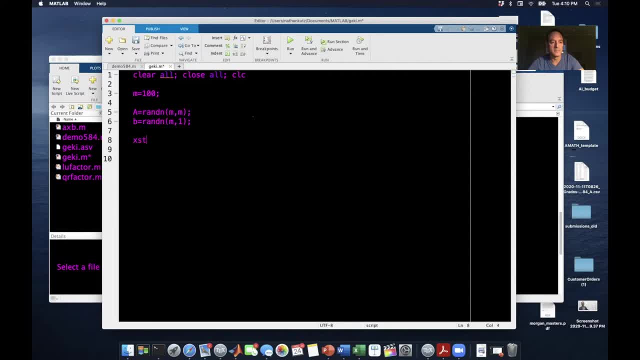 the truth. the truth will be, let's call it x star, which will be a backslash b. okay, so that's my truth, and so i solve this just basically without iteration. it's, i've just solved it exactly. uh, using you know l what, if it's a square matrix, can do lu decomposition and solve that. 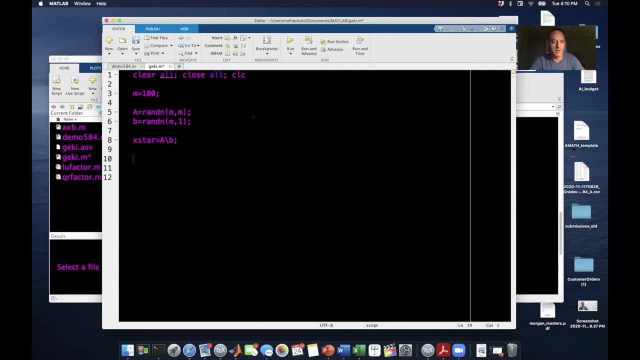 and now what we want to do is solve it with these iteration techniques. so let's call that x. simple as this. there it is done. i have the solution. so, in fact, let's look at the solution and compare it to what the exact answer is. so what i'm going to do is i'm going to make a plot here- subplot. 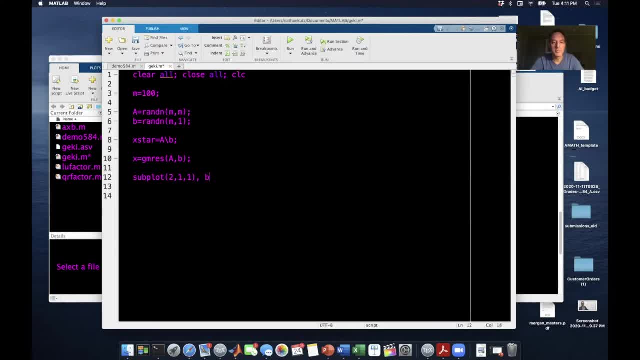 two, one, one, and what i'm going to do here is plot the bar of x star. so this is the values of all the x values of that vector, which is x is a, a vector of 100 components, and that's the truth vector. i'm also going to plot what comes out of gm res. okay, call that x. 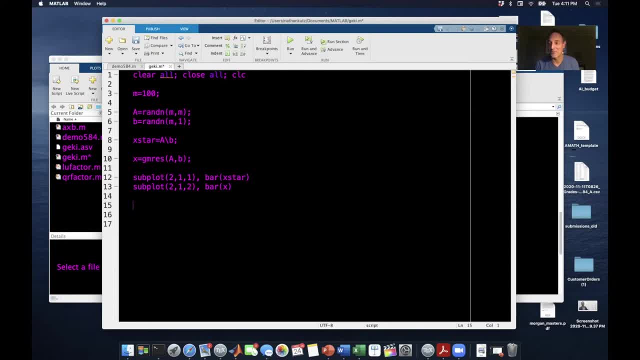 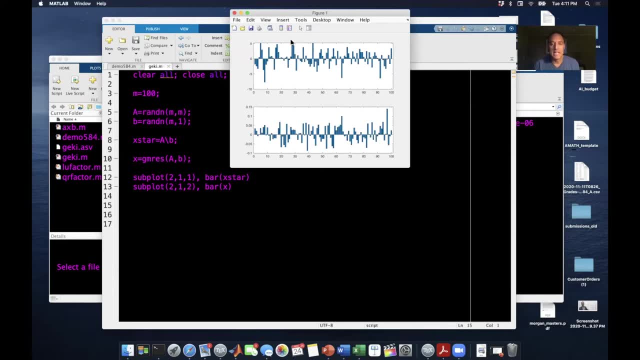 and the question is, of course, that you'd want the solutions to match right. so check it out. i run the solution through all those, and then i'm going to compound, and this equation that i've just made is going to be fined in respect of this. so what i'm going to do is i'm going to 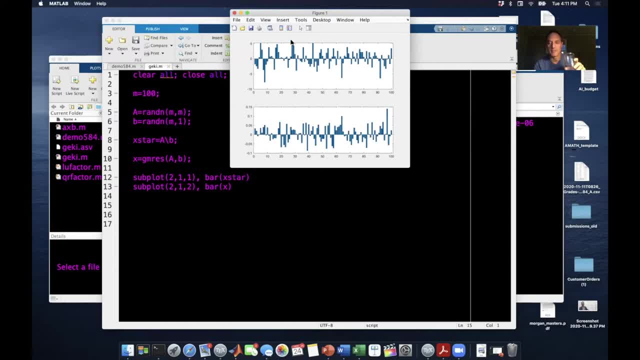 find all the values and then i'm going to put them down into this given function and then i'm going to count them the entire way up to minus one, and so i'm going to find the solution, and i'm going to have to do this, so i'm going to see if the solution works and then i'm going to 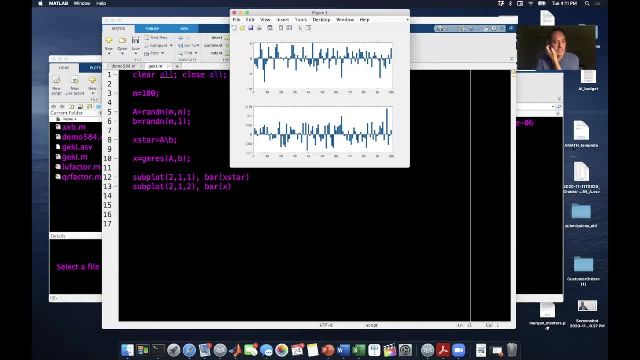 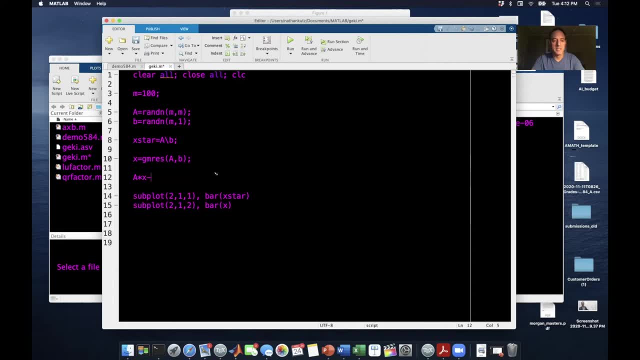 get the number of the original values. so let's talk about that here. this is my first time. I'm also gonna just compute the residual right. I'm gonna say: well, what is AX minus B? Call that R and let's get that number. 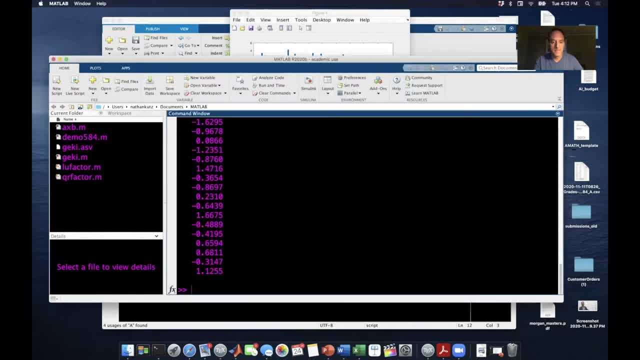 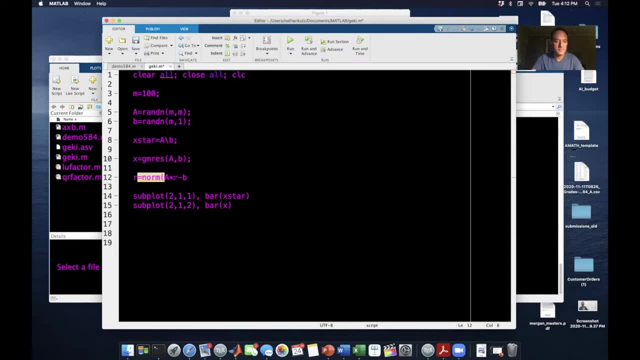 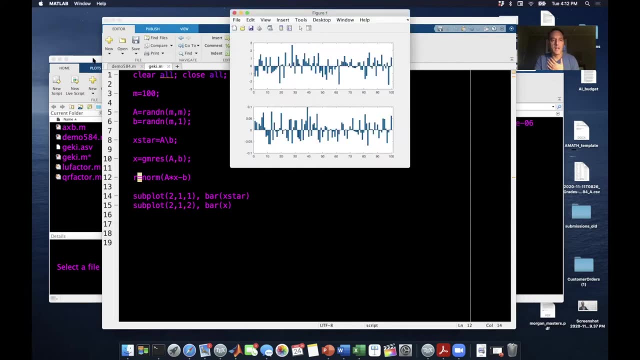 So when I run this, there's that and, oops, I want the norm of this. sorry, I want the norm of the residual. So how big is the norm of the residual? The difference between that and it's pretty big: 10, okay. 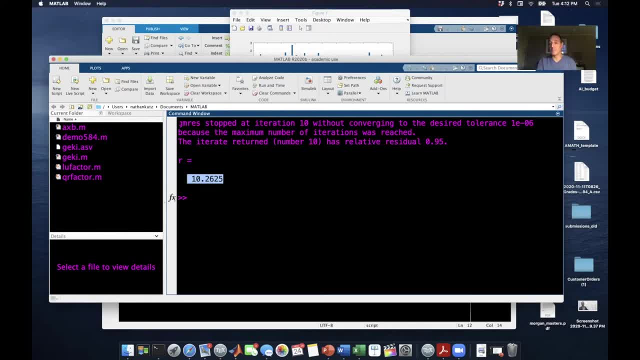 And notice, by the way, it's giving me an error here. So the residual is big, so it's not even close to the solution. And it says: GM res stopped at iteration 10 without converging to desired tolerance of 10 minus six. 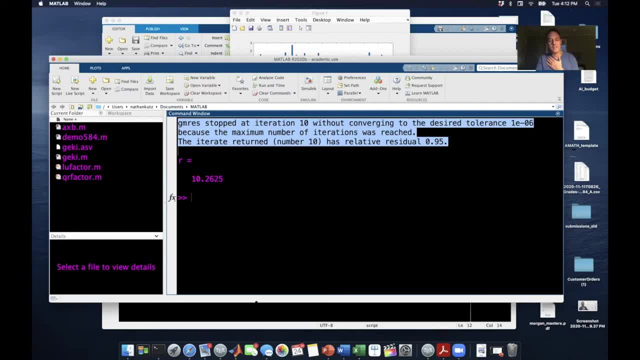 And, of course, it's obvious that it did that. All right, so let's go ahead and take a look at what we can do with this. Okay, so let's go back to help GM res and let's look at some of the options. 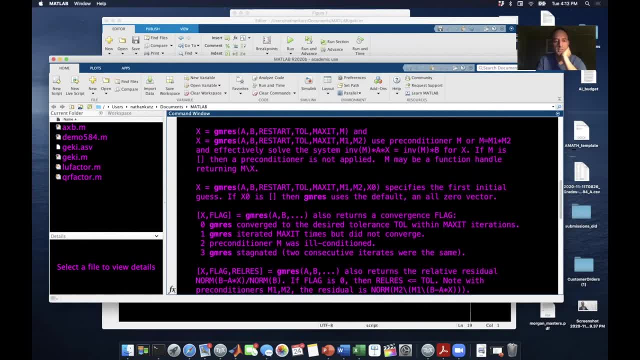 and look at some of the flags. So first of all, if I wanna go through more iterations there, it is right, there it's this component. So I look at A and B. I put an A and B. let's say I don't wanna do anything. 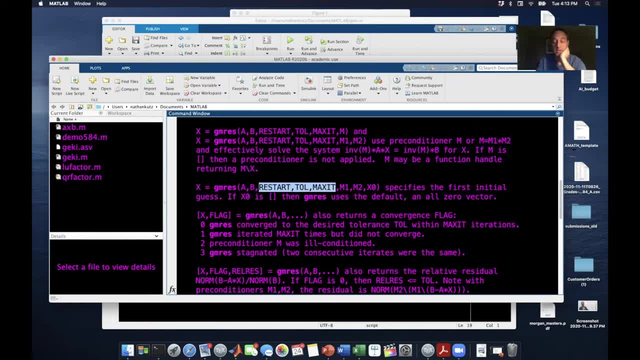 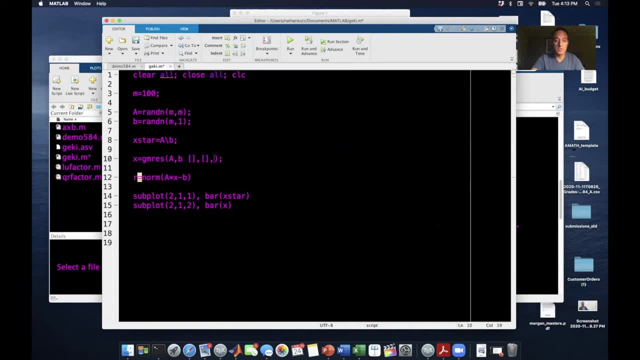 with a restarting the tolerance, So then I would leave those as empties and then maximum iterations. I could put something in so I can do GM res and I put these as empties, which is zero, which is the tolerance right And as well as what was it? 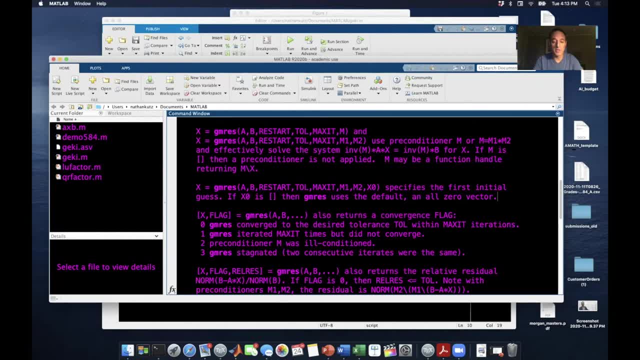 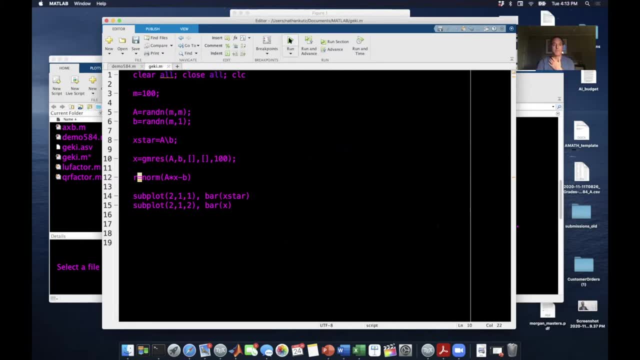 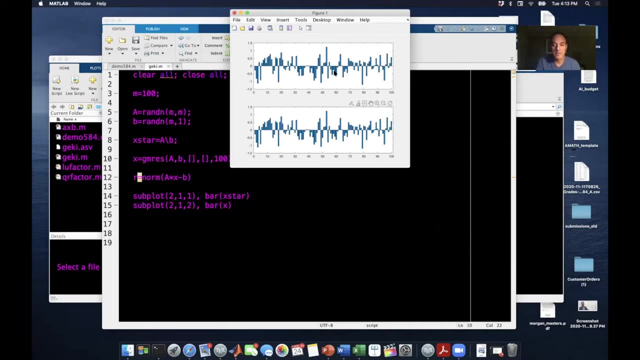 Sorry, it was the tolerance and the restart, And I just tell it here: how about 100 iterations? Okay, so now I'm gonna run this. Okay, so actually that looks a little better, doesn't it? Look at that, these are starting to look pretty similar. 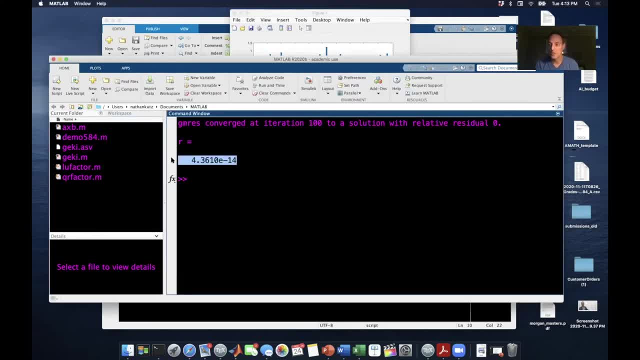 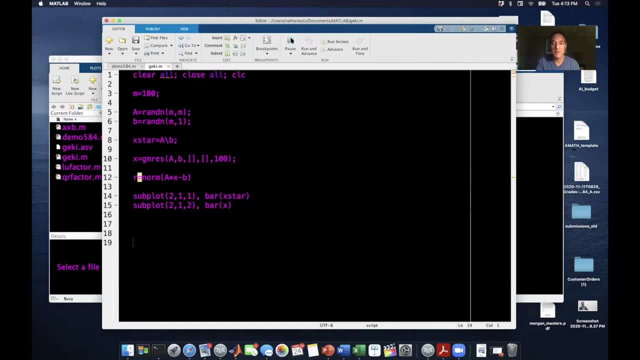 In fact. now check it out, The residual is 10 minus 14.. Okay, so I just needed to iterate longer. Let's do it again. Remember, every time I do this is a random matrix. There we go, look at that: 100 iterations and I got it. 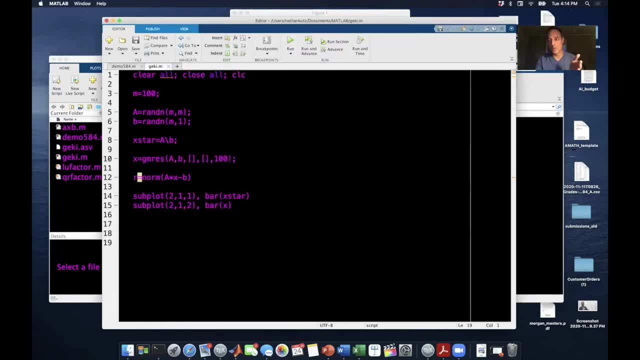 So what happened? Well, now I'm iterating quite a bit more. So, instead of just 10 iterations, which I didn't converge, now I'm doing 100, and this thing is converging. Okay, let's do some more diagnostics. 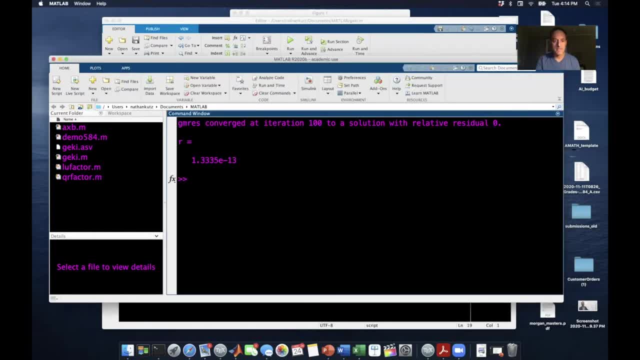 In particular if I come back to here, oops- and, by the way, look at what it says here- GM Res converged at iteration 100 to a solution with residual zero. great, So let's do help GM Res, Okay, and let's pull this thing off. 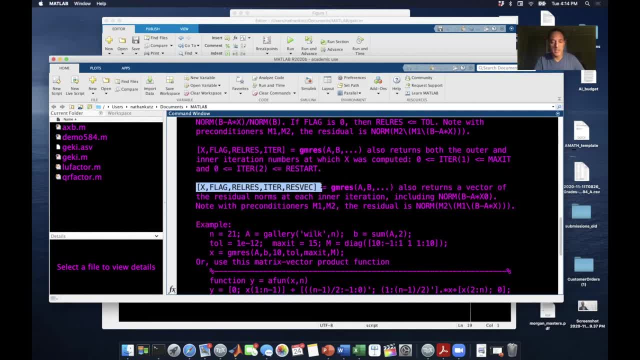 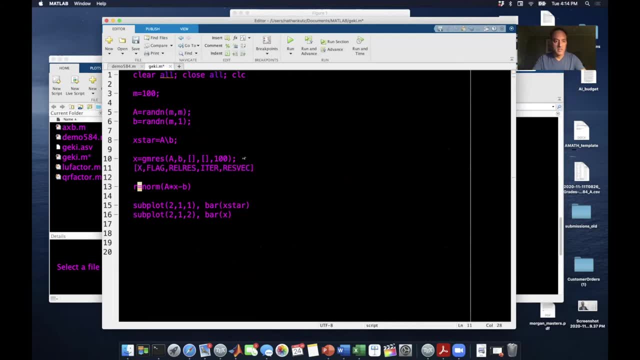 And I wanna start looking at all of this stuff. So I wanna start getting some more diagnostics out. So let's copy and paste this over Here, and I don't like having all of these as let's do this. copy this here and I'm gonna call that X. 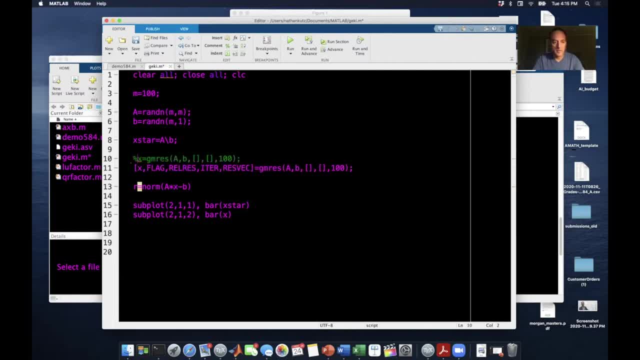 And we'll just leave everything else. capital X, but all right. So now I'm gonna do the same command, but now I'm gonna pull back all of these extra quantities: the flag, the relative residual, the iterations, the ResVec. 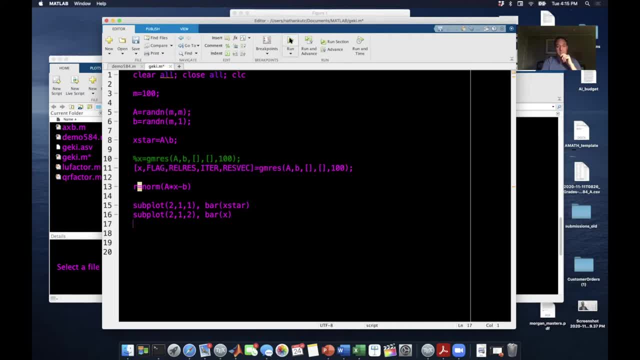 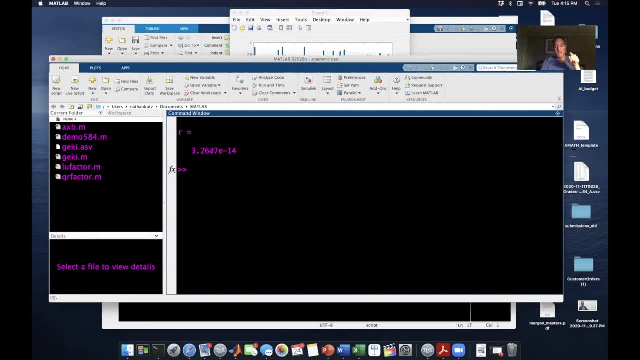 Okay, So I'm gonna run this again, And what we're gonna do is again: take a look, There I am. I've converged to the solutions with 100 iterations. Okay, the residual is 10 minus 14.. And what I'm gonna plot now is make a new figure. 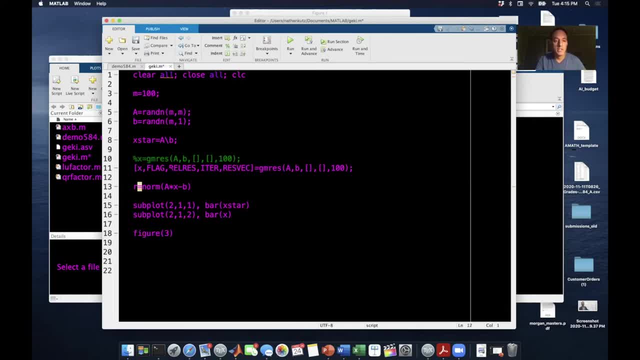 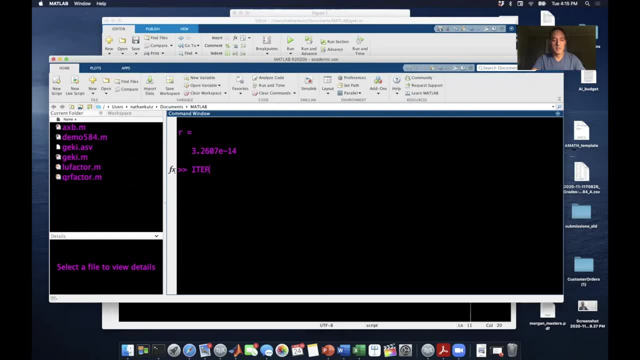 And there's some things I wanna look at. So first of all we can look at relative residual in iterations. So that's gonna be. So let's look at iter first. So it went all 100 iterations, So another stop on the way in there. it just went all the way through to the maximum number of iterations allowed. 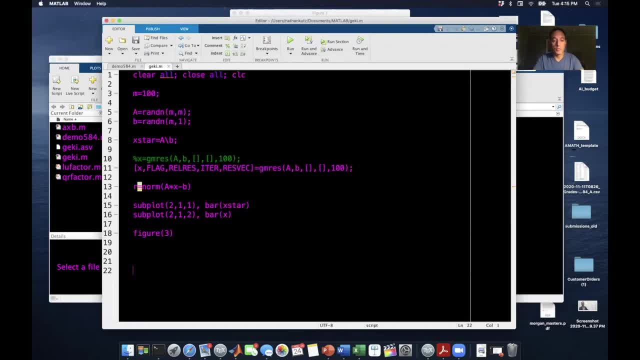 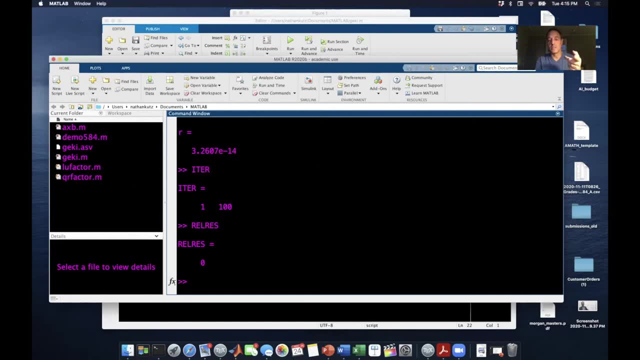 and, by the way, they're rel, uh rel res, relative residual. this is relative residual, not just what i had written down, it's zero. so you know it's not this here. or we computed, which is just how well is it? how was the norm of ax minus b? so a little slightly different measure, but does a pretty. 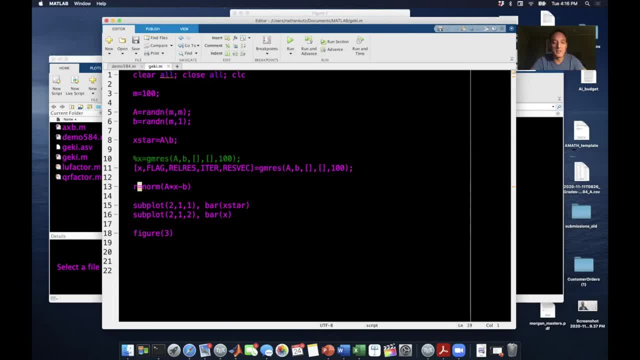 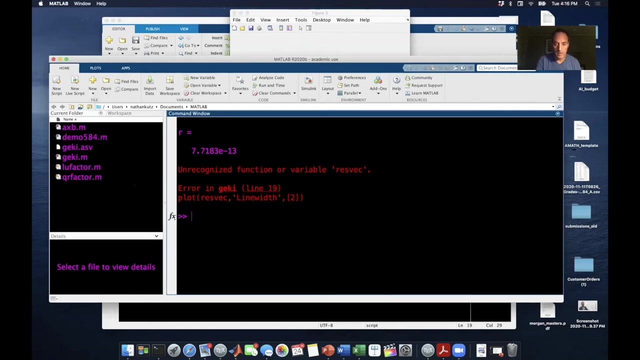 good job. the more interesting one to plot is: let's plot the resvec and let's make that line with two. and so what this is going to show us is this vector of residuals as it's iterating along. oops, oh sorry, it's all has to be capped, sorry. 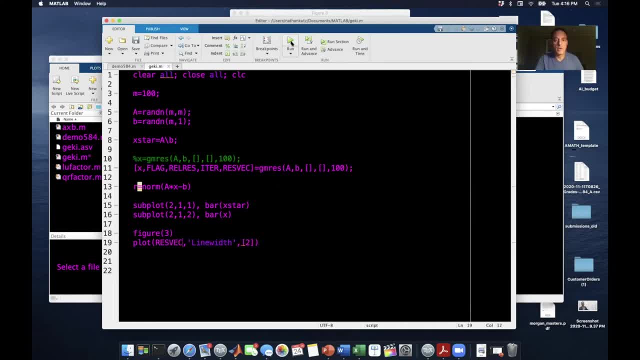 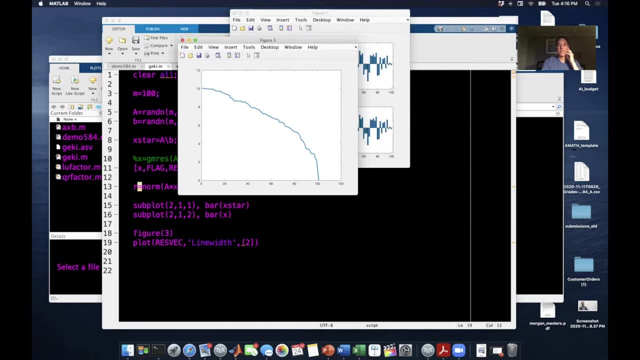 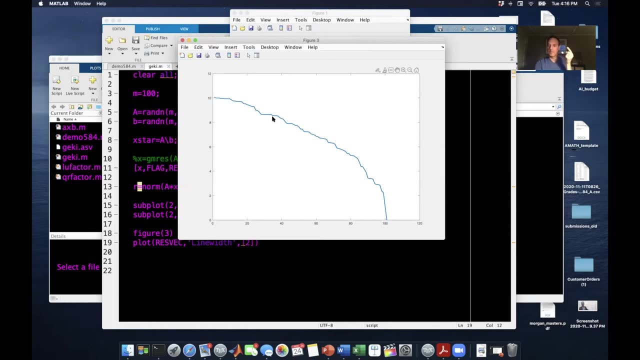 there we go run and there it is okay. so there is what you're seeing. this is how this thing iterated to the solution. so it's an iteration procedure and what you're seeing here is the relative residual at each step of this iteration as it goes through, and notice how it sort of dives. 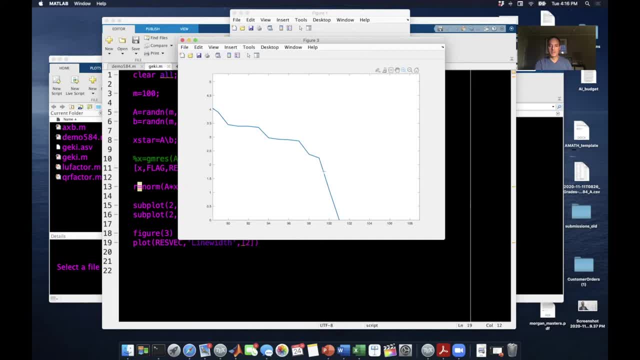 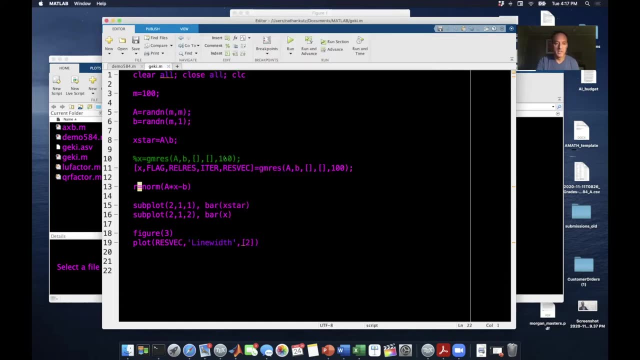 down here around: uh, iteration right at iteration 100, it just pops way down. so remember, i go to 100 iterations, so at 101 is the last iteration and notice how it just basically tanks to zero. let's actually maybe bring this up and say: let's only go through 80 iteration, 80 iterations run. 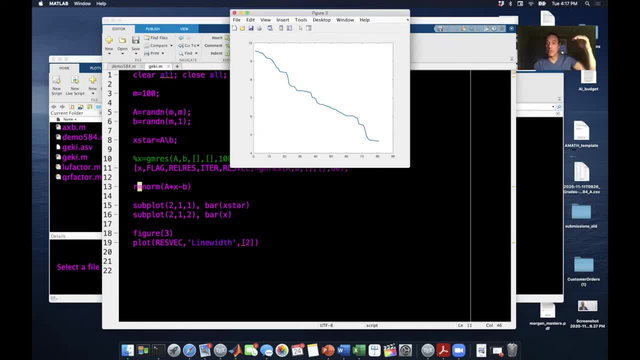 so now look at that. so now it's 80 iterations. notice how the error keeps dropping. so it's finding better and better approximations to the vector x as it goes, and of course here it didn't quite do it right. it took 80 iterations. it's not down as small as i'd like it to be right, or as 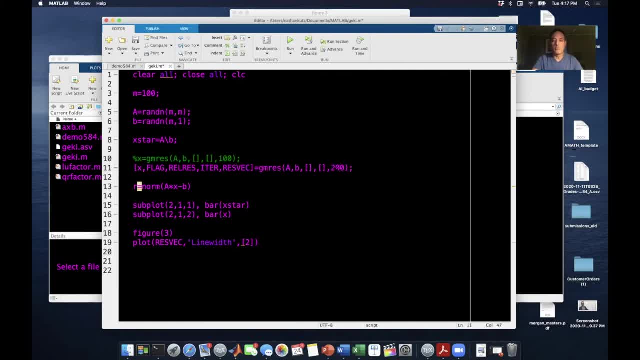 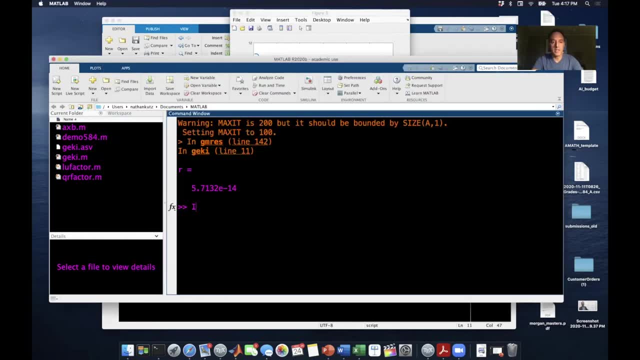 long as small as we'd like it to be, and if we go to 200 iterations then it basically stops here and then we can say iter. so, uh, i don't actually know why. so it stopped at 100 iterations. it seems all right, set max to 100. 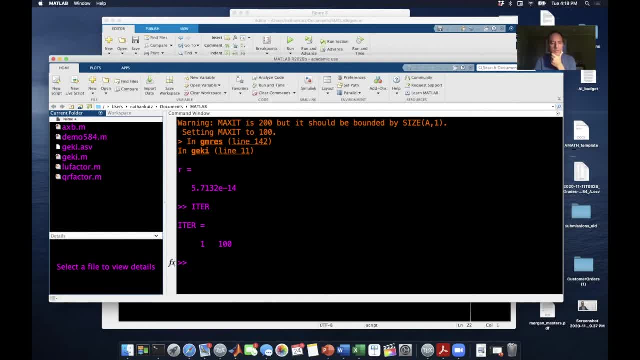 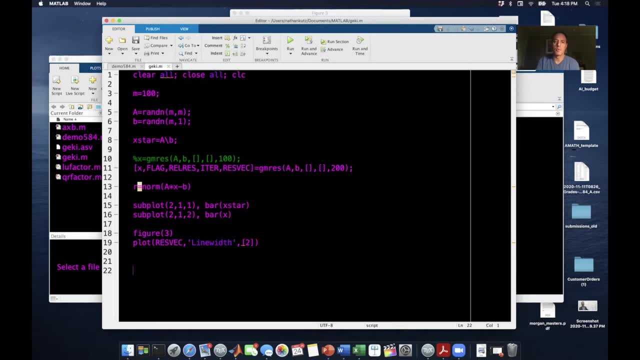 uh, all right, so anyway, the iterations is 100.. so basically it, it basically got the solution uh, there for us, uh, after 100 iterations. now, in this case, it took 100 iterations to get to our solution, right, so it's not necessarily saving us a lot of time. 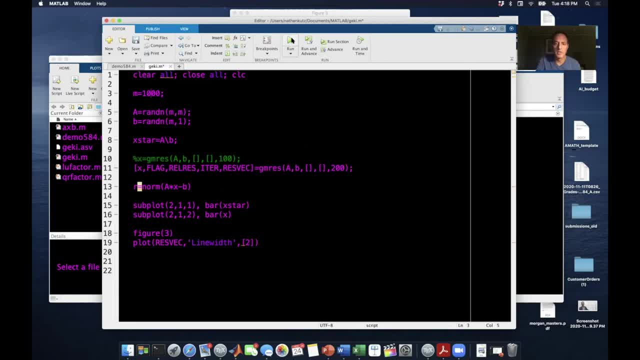 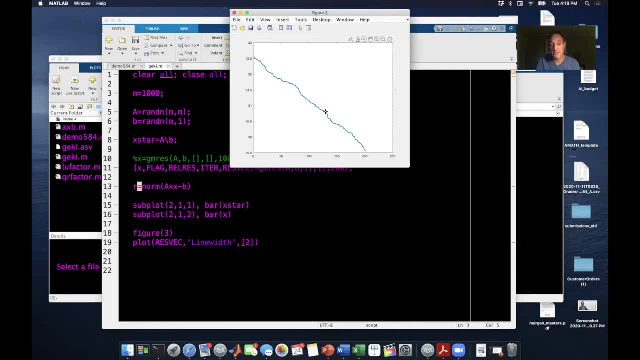 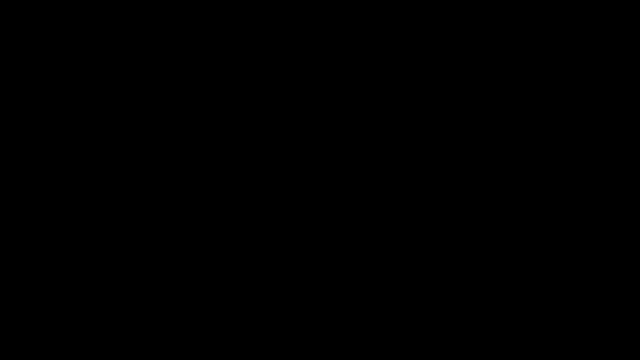 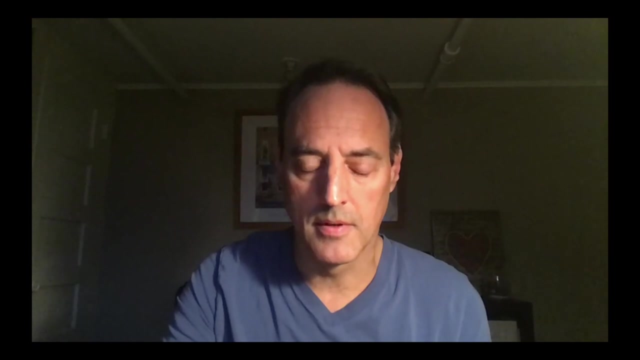 let's actually go up. but here's the deal like when you start doing bigger and bigger matrices: see, now it's, uh, it's taking. look at, this is actually not dropping to zero very quickly, by the way. right, and in fact, the solutions, well, iterations. so all right, let me do screen share again here. 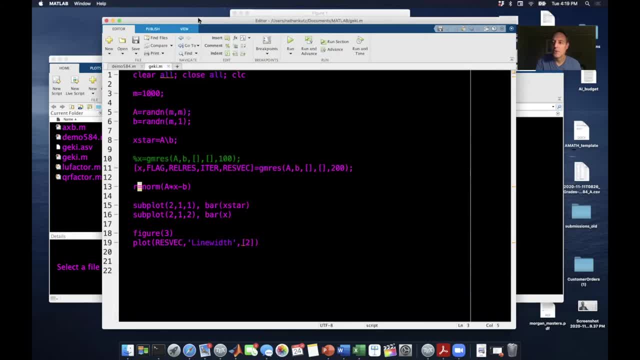 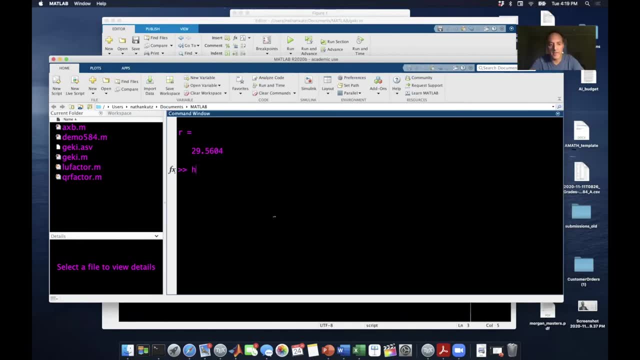 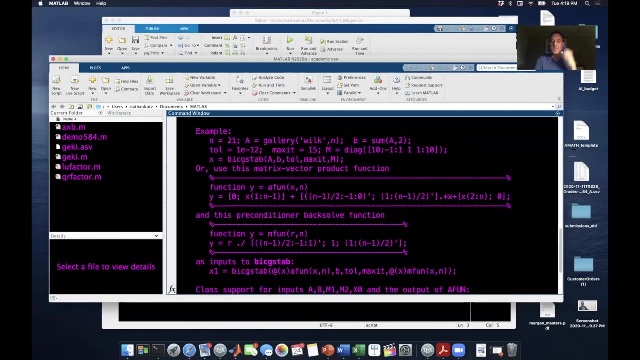 share. okay, i hope this is still recording, all right? uh, last thing we're going to do is we're going to turn our attention now then, so that's anyway. that's enough on that one. let's go to help by cg stab. this is this is the let me. 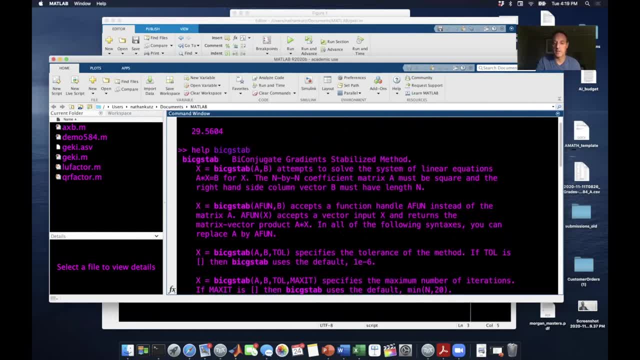 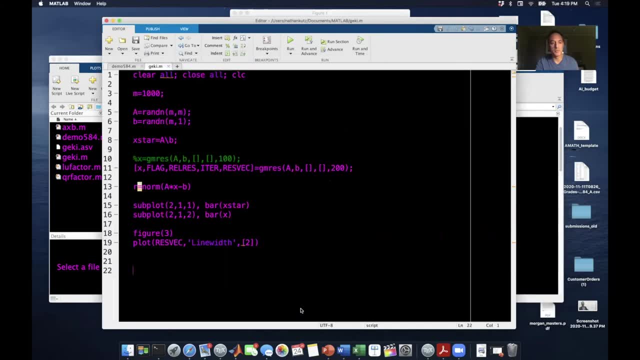 go up here. this is the biconjugate gradient stabilized method, so it's very similar. all you do is replace bcg, gm, res with by cg stab. so basically you're going to come up here and say: x is equal to- let me, uh, pull these out- x is equal to by cg stab, and then you put a, b. so now we can do. 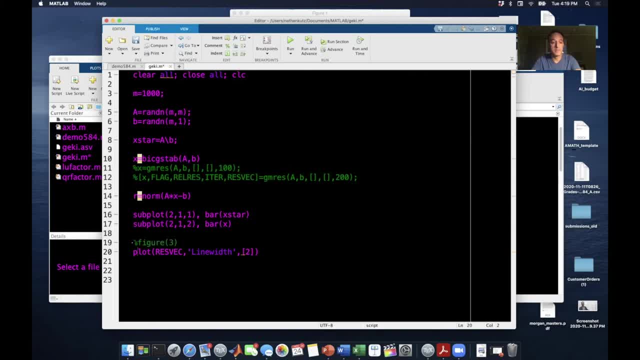 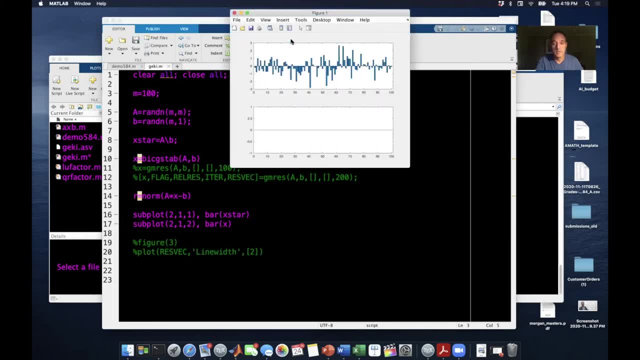 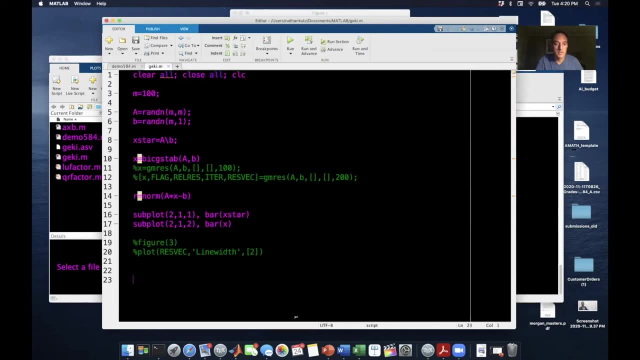 the same thing we did before. i'm going to comment this out and i'm going to bring this back down to a 100 by 100 matrix and let's run it, run it. oops, something went wrong, all right, so why am i getting that thing? 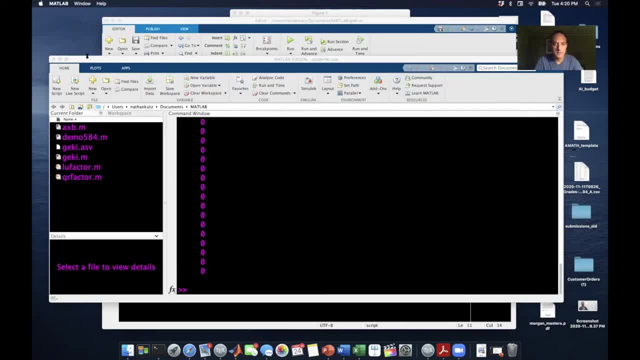 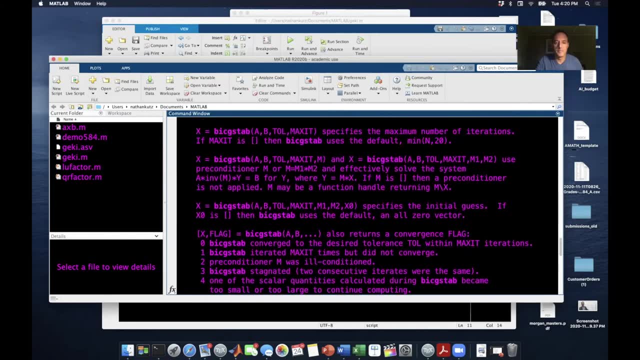 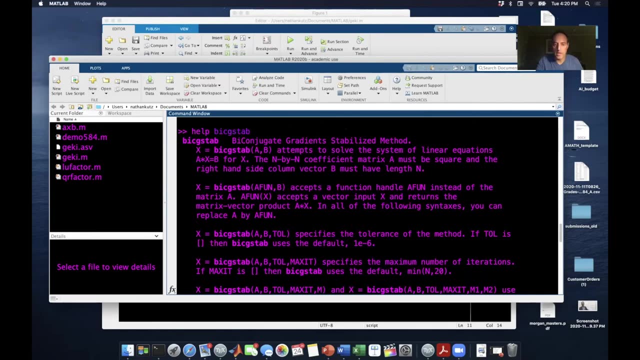 let me go. okay, something's a little funky here. let's go back to read about here and with icg stab right, it's giving you a proxy solution so i can put in the solution. put in a, put in b. it's going to try to go find a solution. 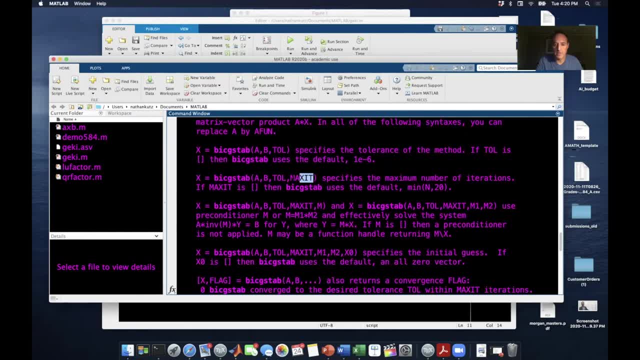 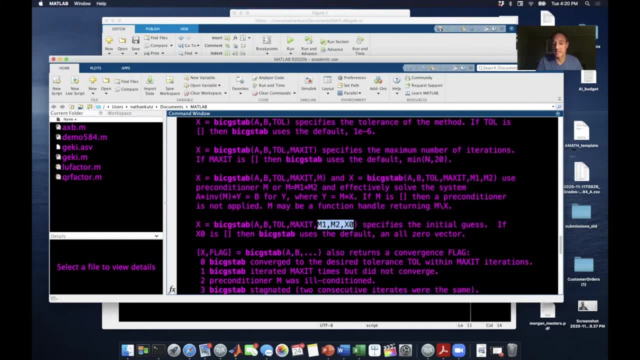 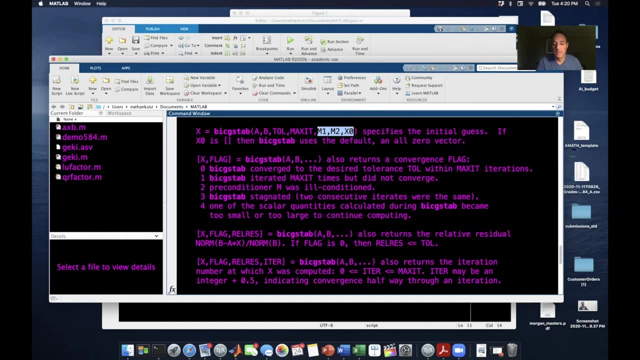 you can specify our tolerance. there is a tolerance. you can also specify its maximum iterations, which is right there, and preconditioners, and also, just like before, you can guess an initial solution, right? so this is the idea behind what you would do with by cg stab. okay, you can pull out all the same things as before, right? 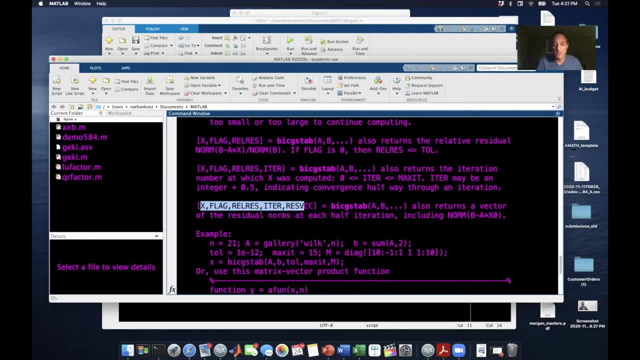 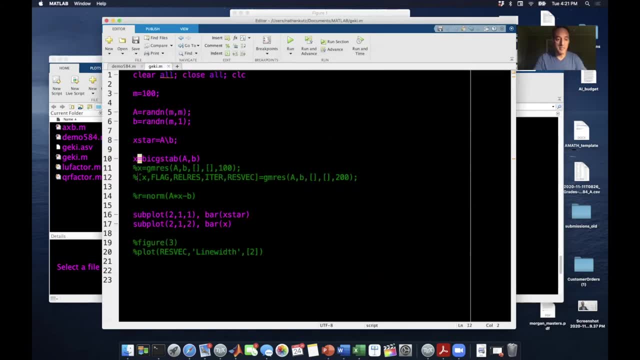 So a flag relative, residual, iteration and resvec. So we're going to pull all those out here where we're going to just basically copy and paste this here And let's just make sure they're all the same: Resvec, iter. so you get flag relative res, iter, resvec. 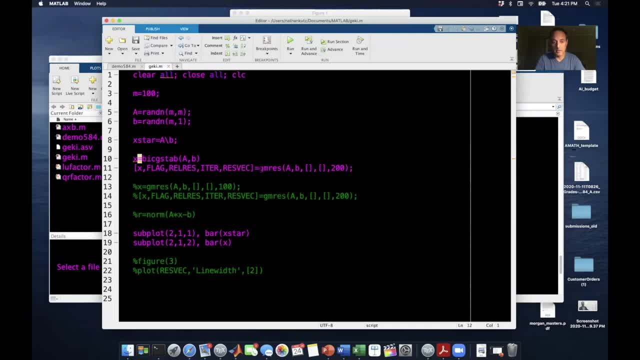 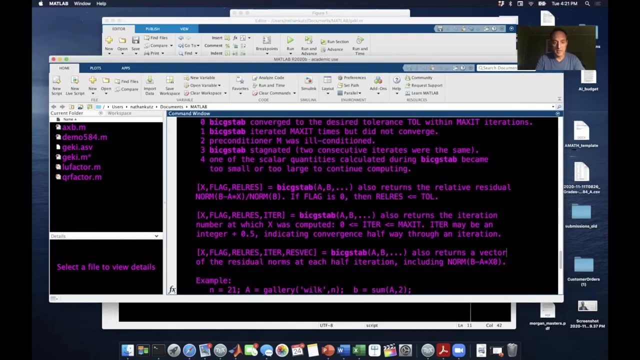 Flag, relative resvec. And then now you say by cgStab a, b and let's go ahead. And now what we want to do is- I think I was giving it, I was actually so- notice that it's a little different. 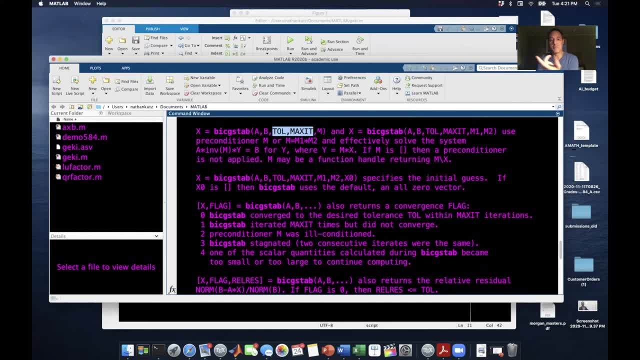 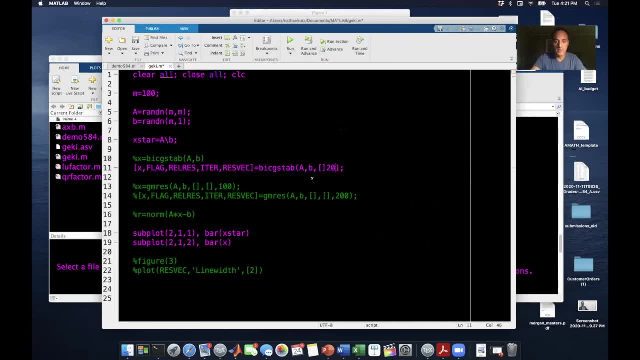 structure, tolerance and max iter, And I had put m to be 200.. So it's probably why it was screwing up. So let's just go through max iter operations 200.. Okay, so we're going to run this. 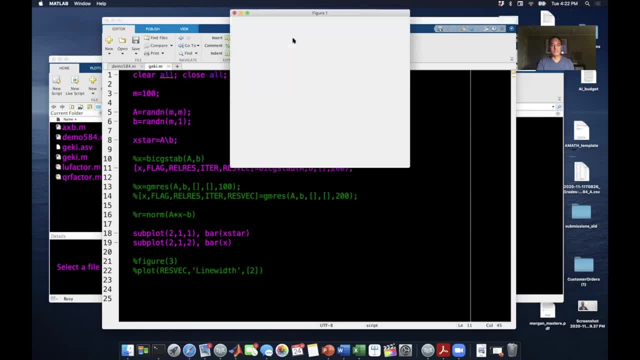 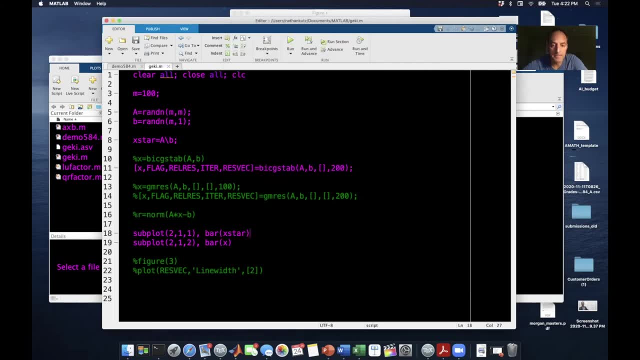 and then we're going to plot our solutions, And this is not making sense. So I'm not sure what's going on, guys. So let's plot this, Let's plot the relative resvec. see what's going on with that. 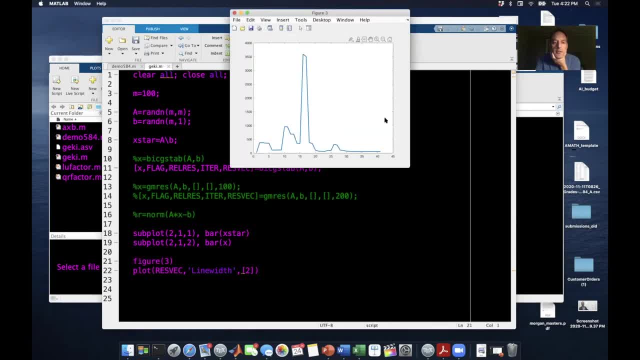 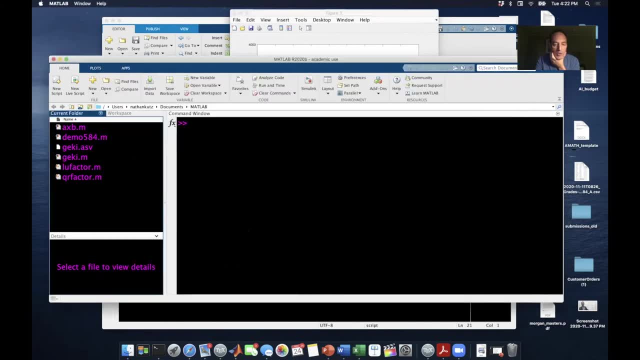 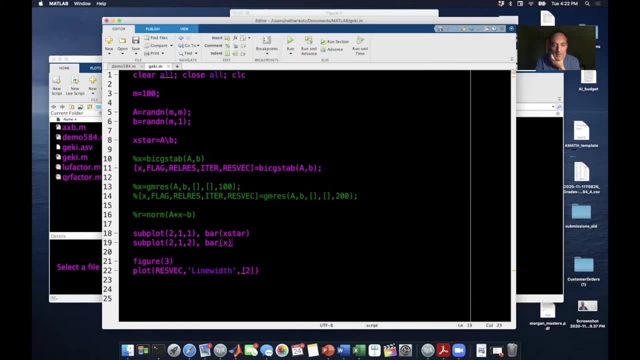 All right. so there's the resvec, So notice what it's doing. And then it's. I think it's actually crashing on us here because this thing here, notice how it goes to 40, some iterations, And I gave it a maximum number of iterations. 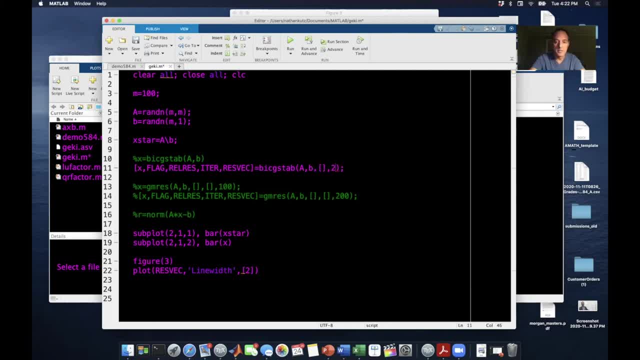 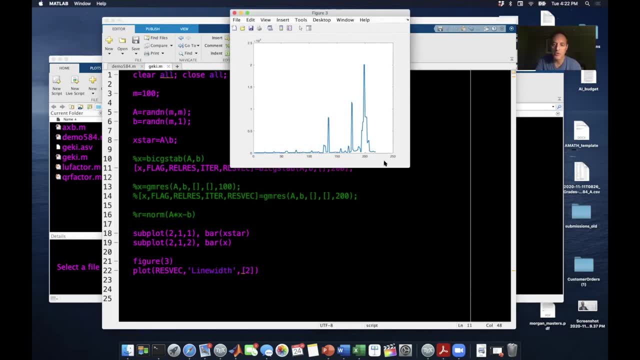 Actually, let's go get that max number of iterations, Let's see. Let's go get max number of iterations, iterations 200. let's run it and see what happens here. so there's the resvec. okay, so there there's a problem. so this, this by g, by cg stab, is not having a good time here. look at this, it's just. 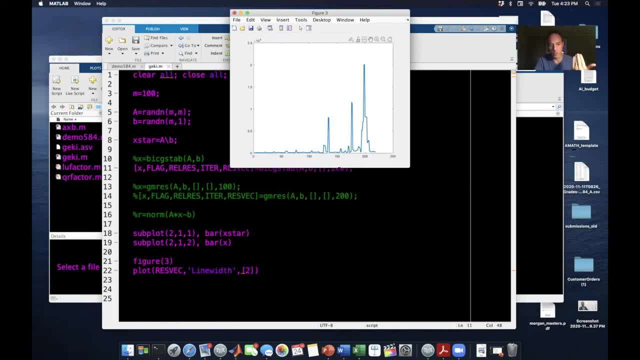 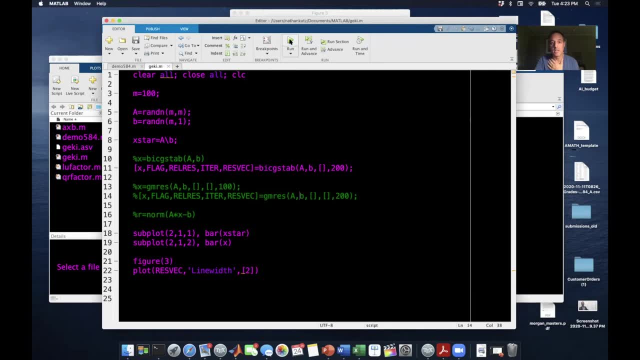 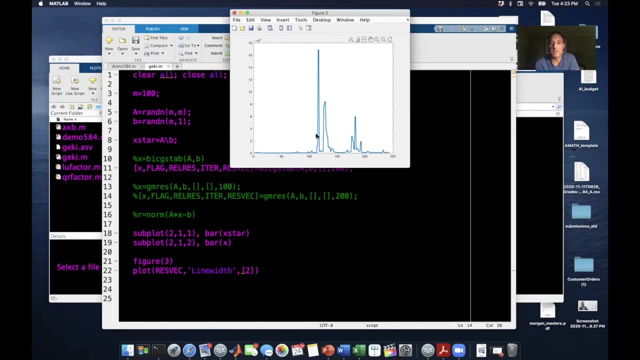 it. this is as iterating. it's actually doing worse and worse and worse. okay, and partly because it's not finding a good direction to search in and get the solution, and so a lot of these algorithms are basically made for certain structured matrices. notice: this is 10 to the 4.. so this is, this is. 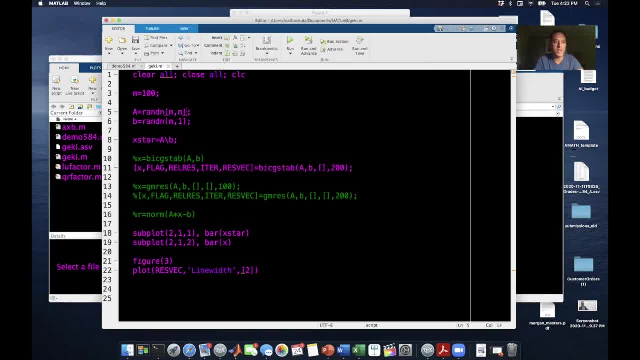 not doing a good job converging at all. so i could take this random matrix a and then add some large diagonal element. so let's do. i m by m, for instance, so that's going to add ones on that diagonal. okay, and still still poor. let's make it larger. see what happens here. there we go see, like i, i made it strongly diagonal. 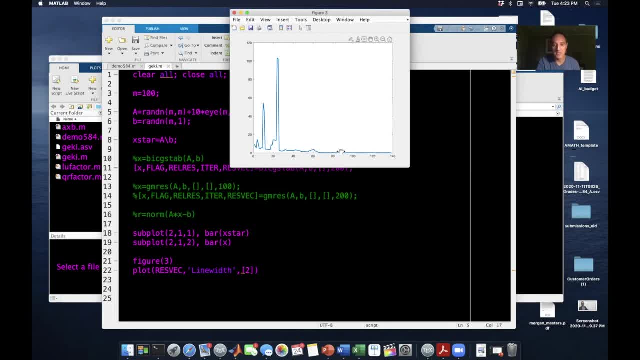 dominant by putting a big diagonal down there and now notice that the solution is starting to converge like this: it just takes these big jumps and if i zoom in here it's starting to converge. so you see that what i just showed you is by cg. stab actually does not work well for just some random matrix, whereas gm res did okay. 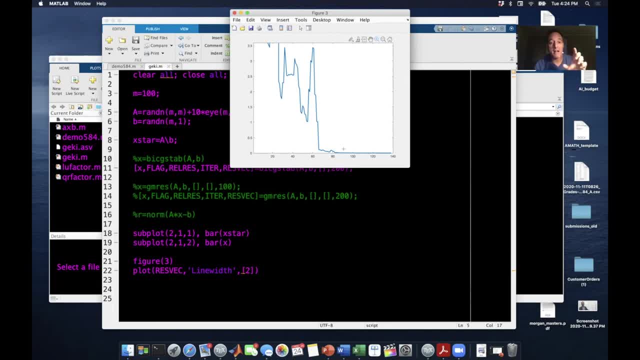 however, by cg. stab is really good when you have some of these diagonal matrices that often show up in computation, scientific computing applications. and there you see what it's doing. right, it does a wiggling around and then it pops in towards the solution and so obviously it doesn't you know. so, in other words, these iteration techniques,